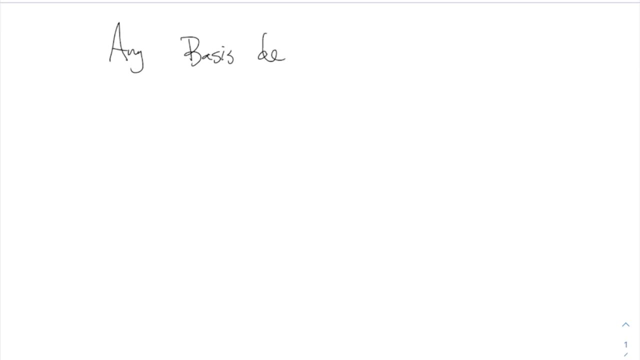 defines a topology. This is the point of using a basis for a topology. Remember, in order to be a basis, a basis means some typically like smaller collection of open sets where, first of all, they have to cover the whole space, That is, every point has to be in one. 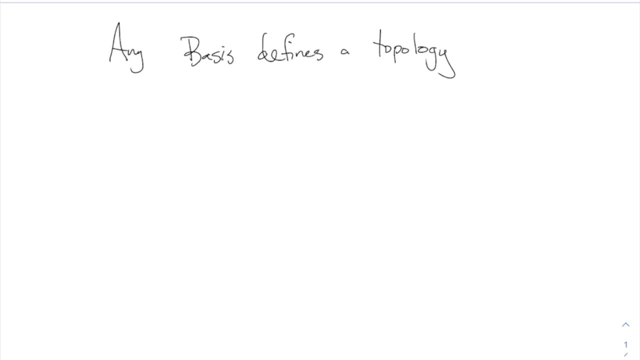 of the basis sets. And secondly, the basis sets have an intersections property. So remember- this is just a little review here- A basis has two. what it means is all the sets from your basis. So that's a basis. B cover X, They cover your whole space, That is. every point in the space is an. 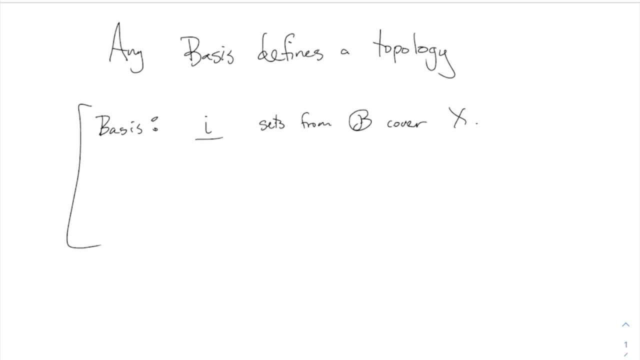 element of one of the basis sets. And then the second thing is this somewhat weird intersections property. It says: if B1 and B2 are basis sets with X in the intersection, B1 intersect B2.. This is what I call the shrinking property, or something like that. It looks like this: If this is one basis, 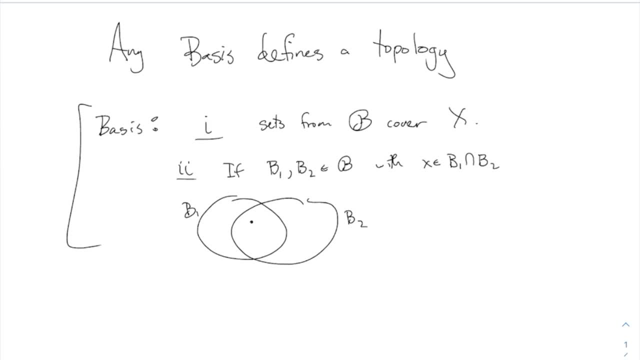 set and this is another basis set. you have to cover X. So that's the whole idea. So that's the basis set and X is inside both of them. then there is a smaller basis set inside the intersection. it means this: there's always another basis set inside the. 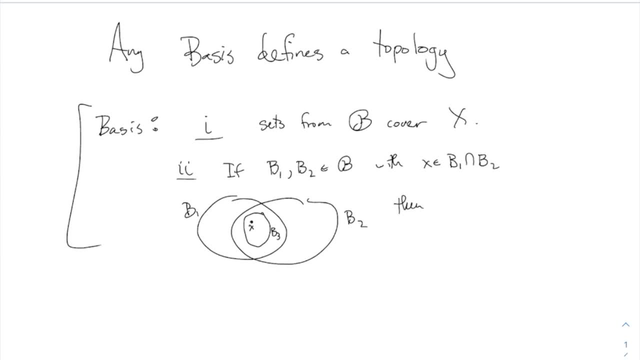 intersection. so the conclusion is then there exists b3. another basis set with X is in b3 and b3 is a subset of the intersection. b1 intersect b2. this is the somewhat strange intersections property that says, whenever you have two basis sets which have an intersection, there is another smaller basis set which is: 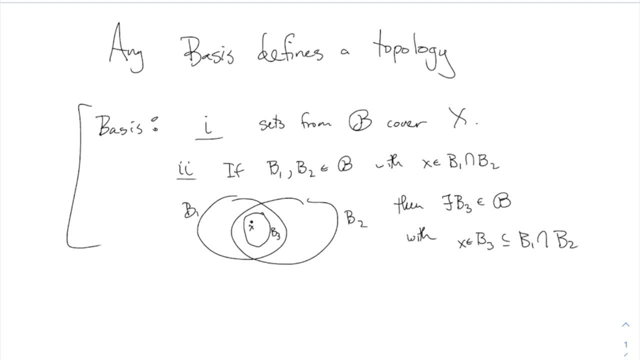 contained inside the intersection. all right, but anyway, the whole point of all this is that any basis defines a topology. for example, the set of all open intervals is a basis, because every element of R is. I mean open intervals in R, because every element of R is part of. 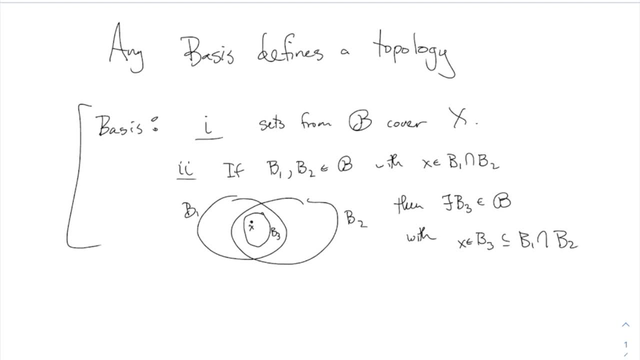 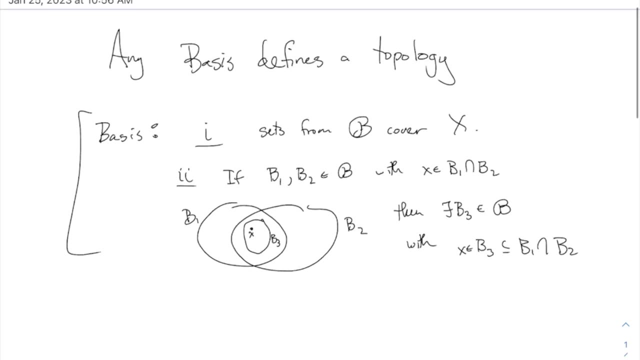 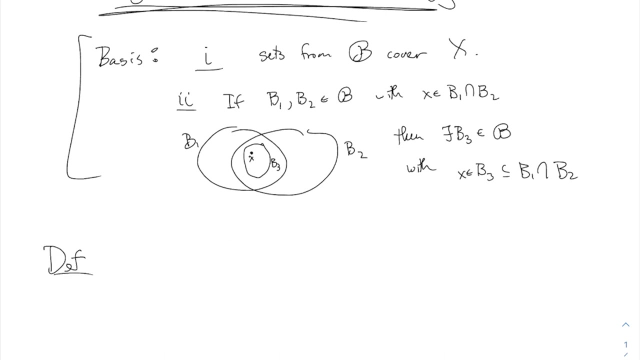 some open interval, and also when you have two open intervals which overlap, there's another little open interval inside the intersection. so the open intervals form a basis, and any basis defines a topology. let's talk precisely about how that works. it's not I've said this several times, but the entire. 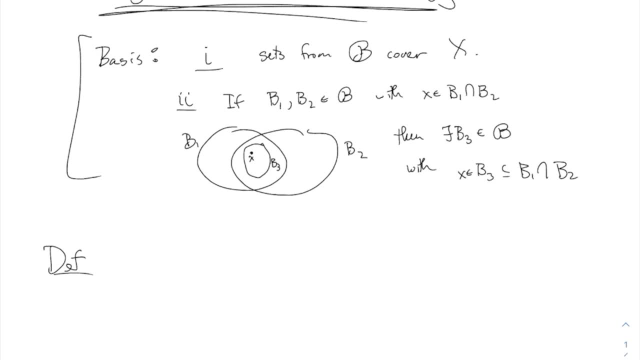 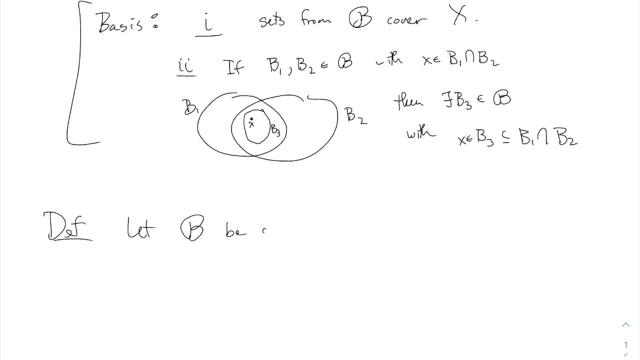 topology is defined to be the union of all the basis sets, or the basis sets together with all of the unions of the basis sets. so I'm going to say let B be a basis, that is to say it satisfies those two properties, the two properties, the two. 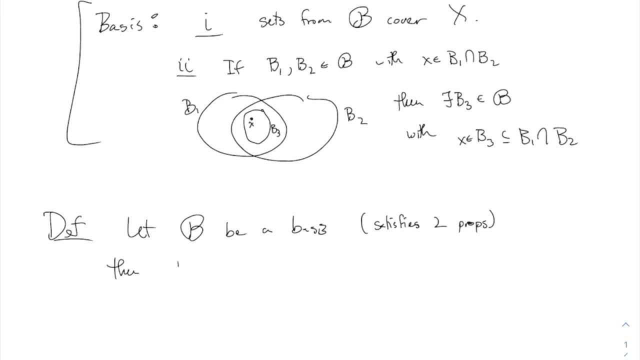 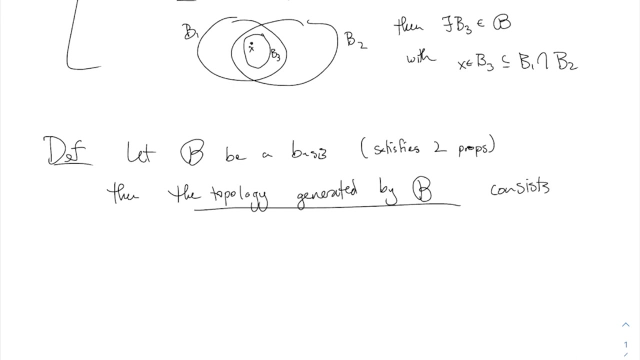 props, then the topology generated by B is the topology which consists of- basically, it's all unions of everything from B, although you also have to, just for technical reasons. every topology must include the empty set, and the empty set is not a union of things from B, So it consists of the empty set together. 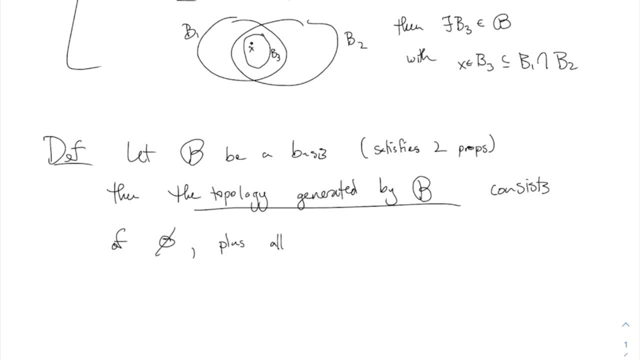 with all unions of sets from B. All right, so this is called the topology generated by B. So whenever you have a basis, that basis can be used to create a topology by just using all possible unions You might wonder about. well, what about intersections? The whole thing. 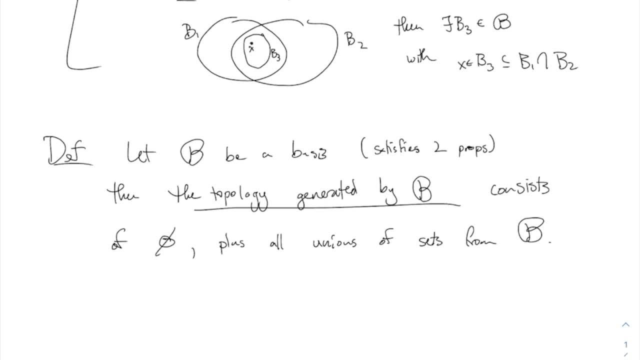 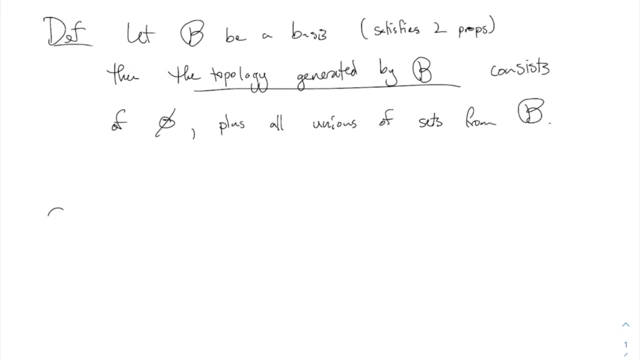 about topology has to be closed on our finite intersections. This weird intersections property here makes sure that intersections will always behave correctly when you're making a topology out of a basis. All right, this allows you to describe many different topologies topologies very easily. So, for example, on the real numbers, if B is the set of all open intervals, 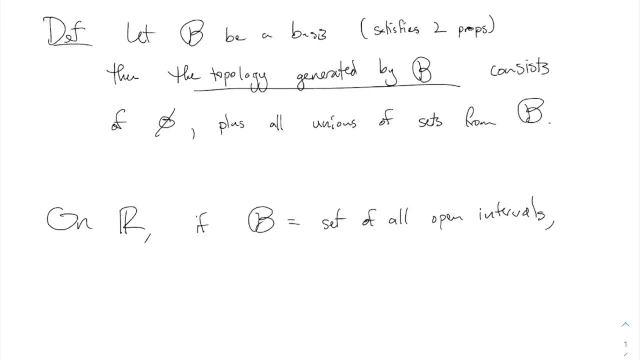 this generates a topology, and this, what it generates, is the standard topology on R. That's what the standard topology is. It's the. it's the topology where every open set is a set of all open intervals. So, for example, if B is the set of all open intervals, 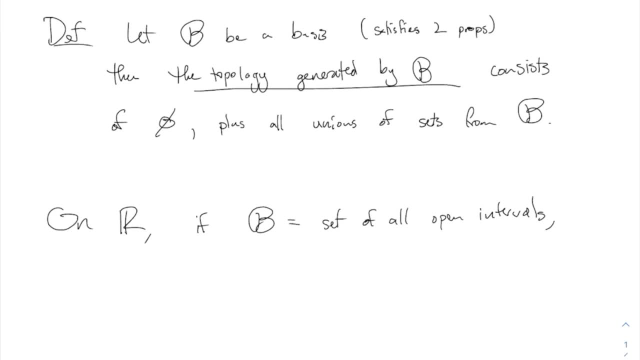 that is a union of open intervals. So, on R, if the basis is the set of all open intervals, then B generates the standard topology. All right, but we could use another, we could make another basis and that might generate a different. 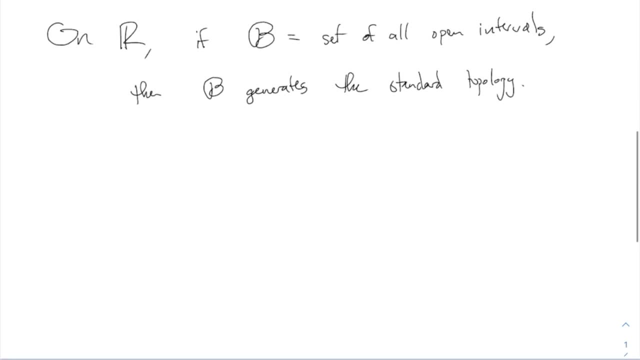 topology on R. So here's another important example that we're going to be talking about. We've already talked about a few different topologies on R. The important ones is the standard topology, of course, but there's also the finite complement topology, which comes up every so often, and there's some 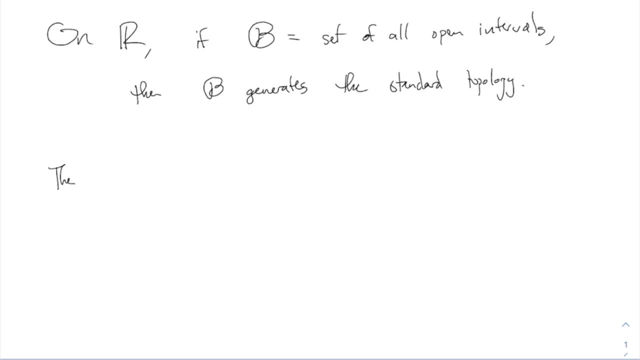 questions on the homework about it. Here's another one: The lower limit topology. you let B be the set of so, instead of taking the set of all open intervals, you let B be the set of. so, instead of taking the set of all open intervals, I'm going to take the set of all. 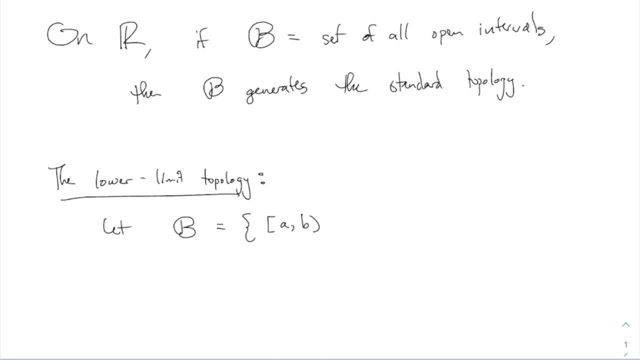 intervals like this which are opened on one side. All right, this is why it's called the lower limit topology, because I'm considering only intervals which include the lower endpoint but not the upper endpoint, All right, and I'm going to call those the basic, the basic open sets, and then any 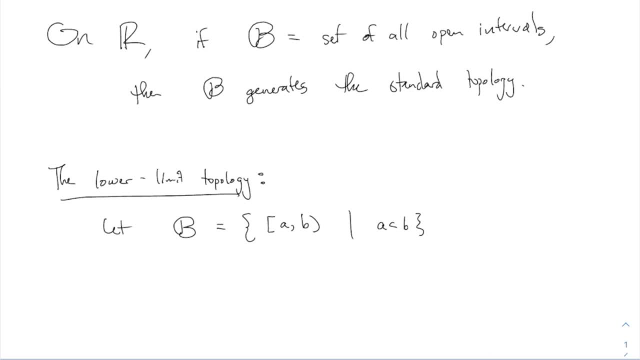 open set will be a union of all open intervals. So I'm going to take the set of all open intervals and then any open set will be a union of things like that. All right, so this is a basis, You know. 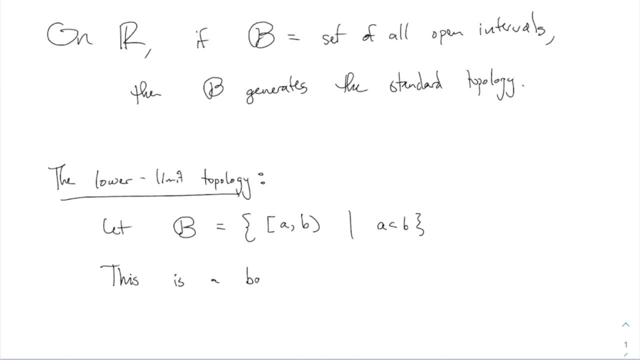 that only works if the thing actually really is a basis. So can we just verify first of all that this really is a basis? First of all, is it true that you know there's the two properties? The first is that this actually covers all of R. Is it true that every real number is part of an? 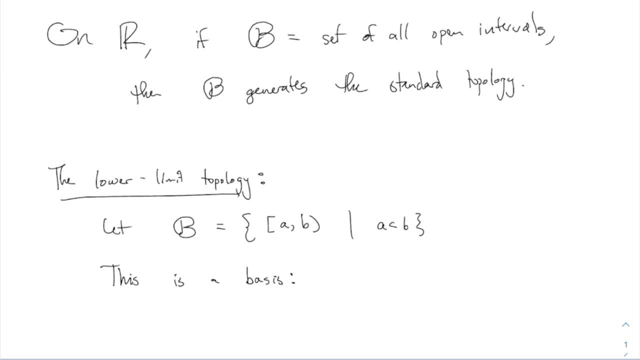 interval like this, which is closed on the bottom. Yes, every real number can be part of some interval like this. So any x in R, as x is an element of you know how about x, comma, x plus 1, right, So every x, every real. 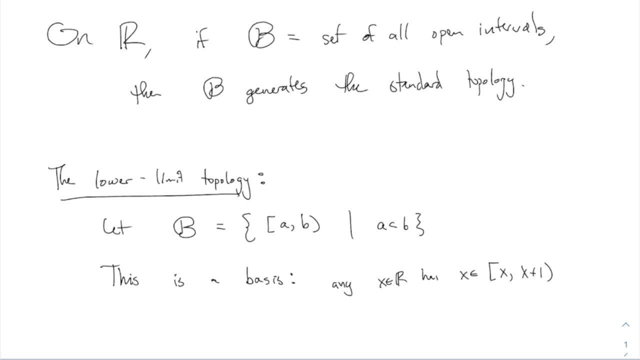 number is actually part of some interval like that, with its lower endpoint included. That was the first property: right of being a basis. The second property is the intersections. Maybe I'll just sort of draw a picture to try and convince ourselves of the second property. So let's say that I have 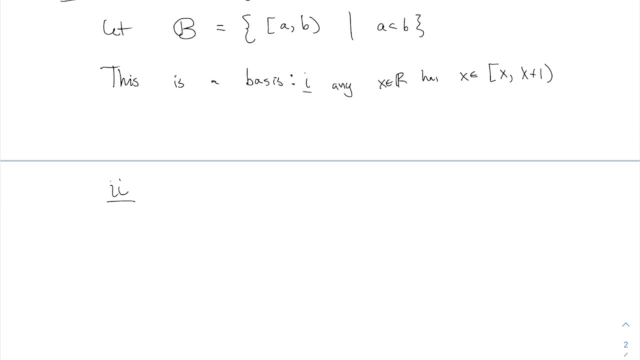 two basis intervals, that is, two intervals which include their lower endpoint and they intersect. They have to. they would look like this: Well, I'll give them names: B1, I'll call A1, B1.. B2, I'll call A2, B2.. And if I were to draw two of these which have some intersection, that means: 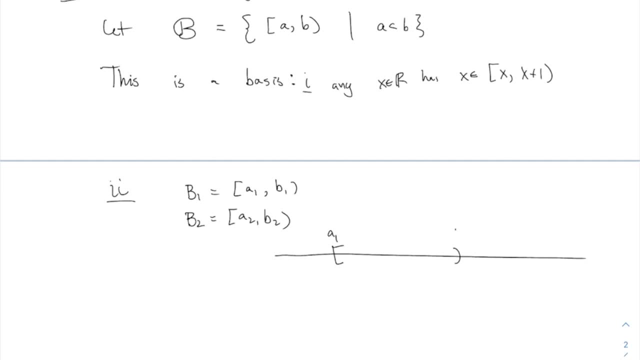 one looks something like this: A1, B1,, like that, And then the other one apparently looks like this: A2, to B2. And they have some intersection where, let's imagine, that x is in the intersection. Now, is it really true that you can put another one of those intervals? 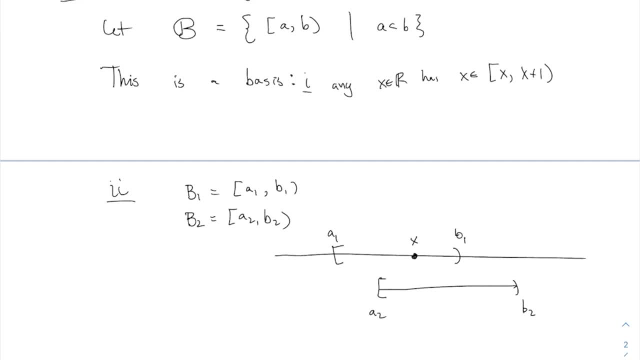 including the bottom endpoint but not the top endpoint inside the intersection. Can you find another one of those intervals that's contained inside the intersection? You know the intersection would be like this region here. right, I think you can. Can somebody tell me? 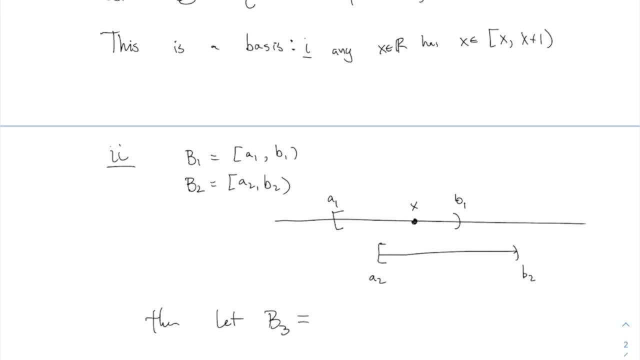 Then we can say specifically: what is the interval which lives inside the intersection? Yeah Yeah, the interval from A2 to B1, including A2, all right, And that has the basis property, that, or the intersection's property that we want. So I'll just 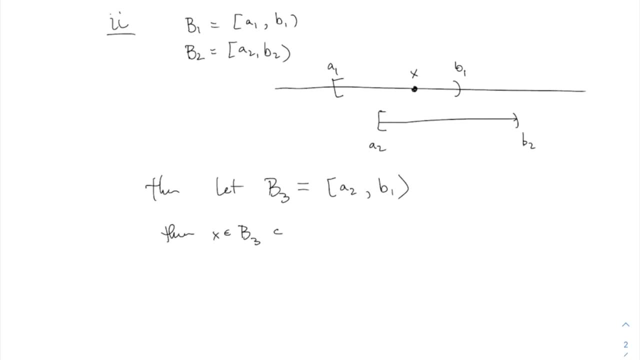 write out: x is in B3, and B3 is a subset of B1, intersect B2.. All right, So choosing only intervals which include their lower limits but not their upper limits, that actually also makes a basis, which means you can use this to make a topology, and that's called the lower limit topology, All. 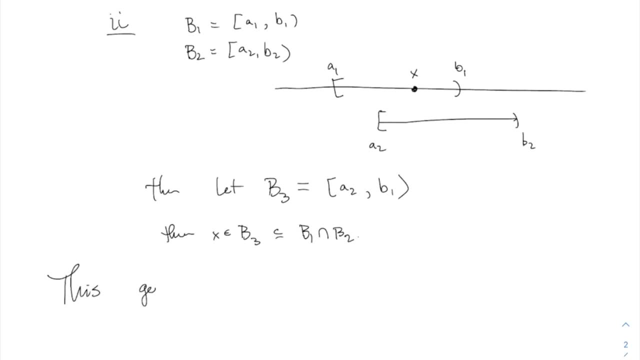 right. So I'll say this generates what we call the lower limit topology on R. All right, The lower limit topology is, in my opinion, quite weird. Open sets in the lower limit topology look like intervals which include the left endpoint. 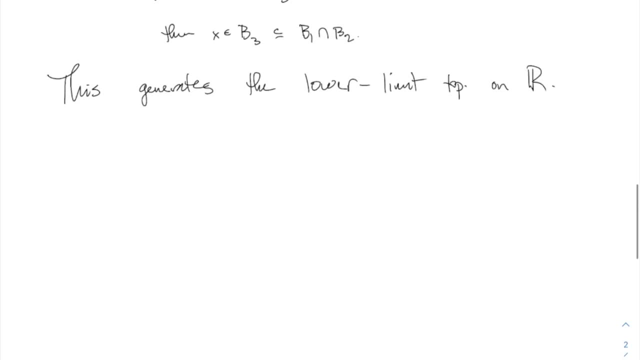 But actually you can get some other weird open sets in the lower limit topology, So in: oh, can I just say: parents here there's nothing actually special about using the endpoint on the left. you could also instead use the endpoint on the right. so I will just say: 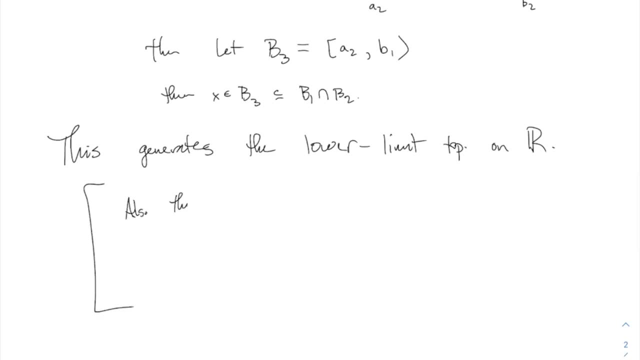 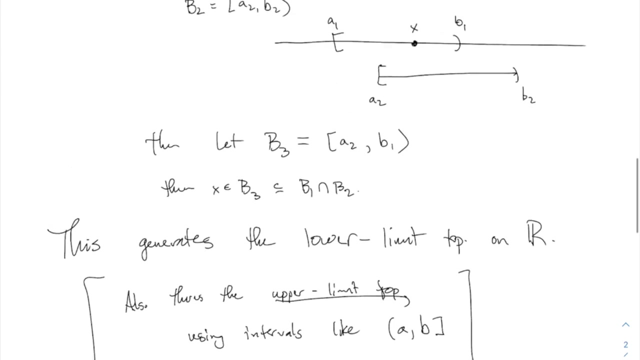 parenthetically. also there's the upper limit topology, the upper limit topology using intervals like a to B, but it includes the upper endpoint. all right, that also is a basis. I mean the same, just sort of mirror image. this picture and you'll see the intersections property also holds for intervals like: 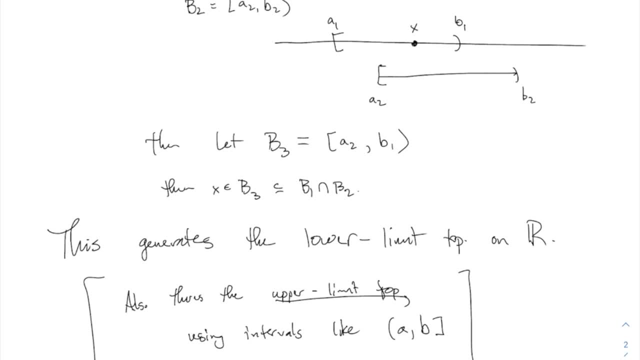 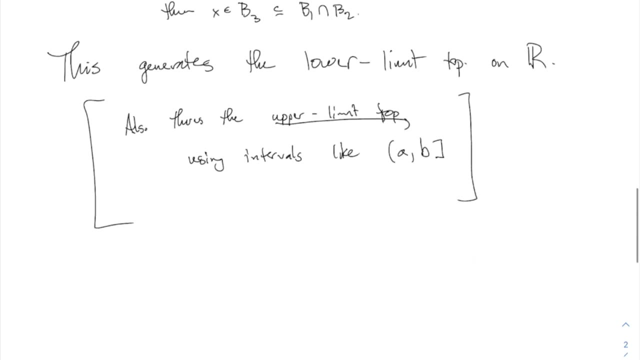 that all right. I was gonna say: what about the lower limit topology? the lower limit topology is quite strange, because so in that was just parentheses with basically anything that you say about the lower limit. the same thing is true, but flipped around for the upper limit. so we're not going to talk about the upper limit. 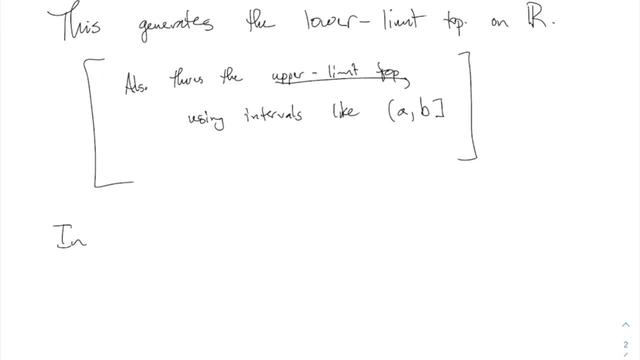 topology very often, but it's it's just as interesting as the lower limit in the lower limit. topology on our open topology, on our open topology on our open sets. well, can I just say something like you know, zero one like this is open right. also, any unions of sets which look like that are open sets. so that means 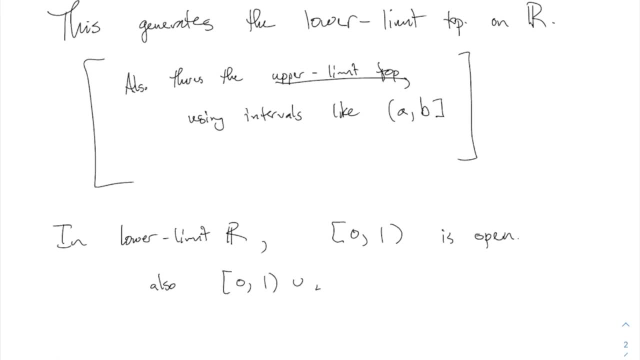 something like: you know, zero, one union, two, three is open, right or any, you know not. just fine, that's a finite union. I only took two sets there, but any, in fact infinite union can be also open. but that means also something like: check this out, I can do: the union of n equals 1 to infinity 1. 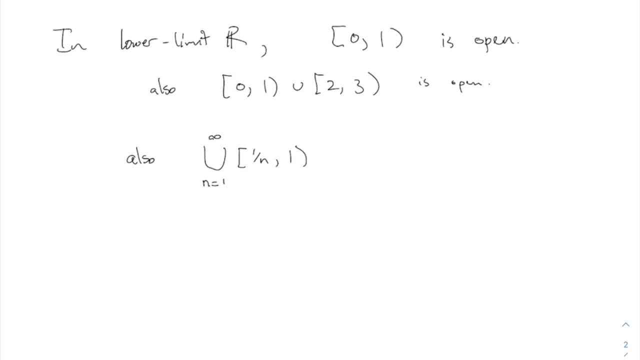 over n to 1. let's say, maybe I shouldn't start. if you start with 1 here, then that that's kind of the empty set. I'll start with 2, just so that I don't have to worry about what does it mean to say 1 to? 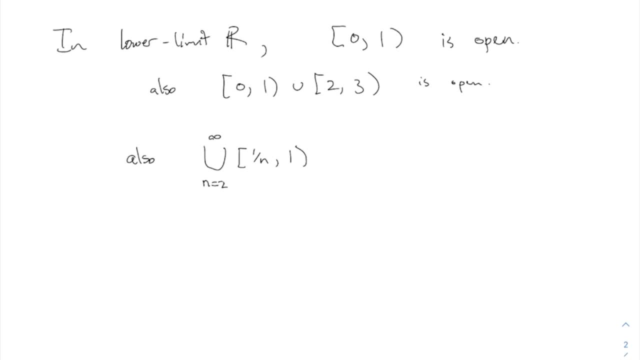 1. close on one side, open on the other side. that's not really a thing. but this is also open, right, because it is the union of a bunch of the open sets. so this is also open. can somebody say that? what, like? what is this? I mean? can we? 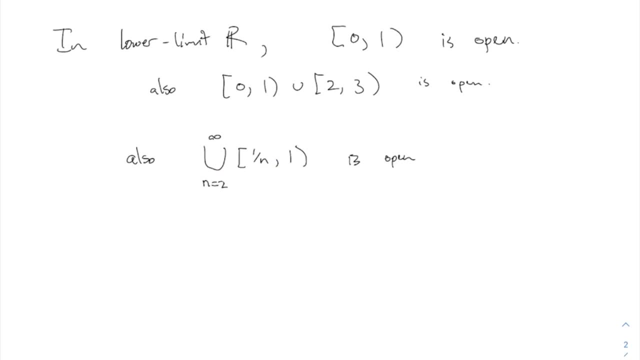 simplify that it's one: the interval 1 half to 1 union, the interval 1 third to 1. if I were to draw a picture of these, if here's one, let's say here's 0, 1 half to 1 is here right, not including 1, and then the next set in the union is 1 third to 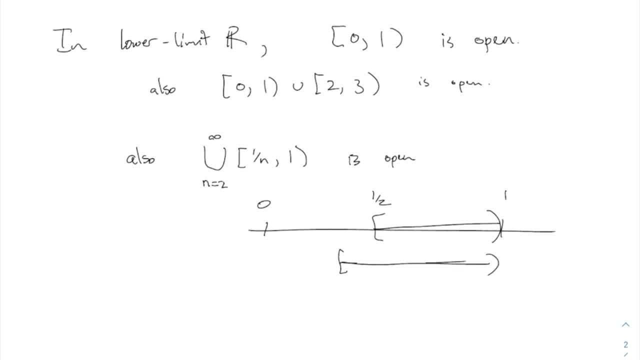 1, that would be here. the next set would be 1. fourth to 1, which would be here. I'm taking the union of all of those. what is it? what do you end up with? yeah, it's the open interval from 0 to 1. yeah, this, these intervals, actually, eventually they. 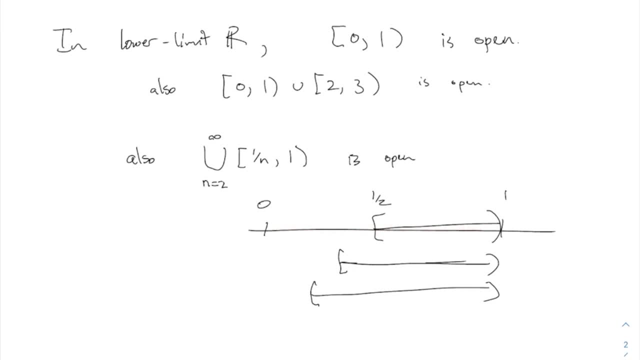 they, they cover this entire thing but you never actually get 0. but you do get all numbers approaching 0, I suppose because of the Archimedean property- remember that anyone taking the comp this weekend- because numbers like 1 over n approach 0. so this is why I said this is very weird. 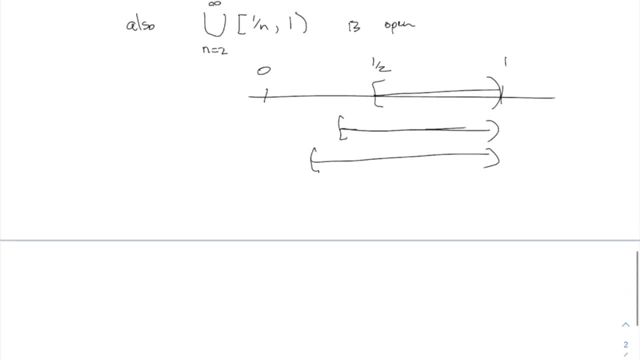 in. this is open, so that means this union. here. this actually equals the open interval 0 to 1. all right, so in the lower limit topology on R. the moral of the story is: this is open and also this is open, pretty strange. so an open set would be one which includes its lower limit, but also like 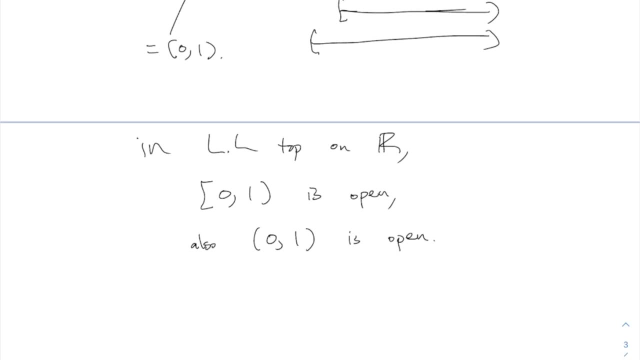 if you allow those to be open, then automatically the ordinary open intervals are also all open sets. so actually this is a finer topology than the standard topology, because every standard open interval is also open here. but this has some some more stuff is also is also open. all right, very strange, you might wonder. maybe it maybe everything is open. 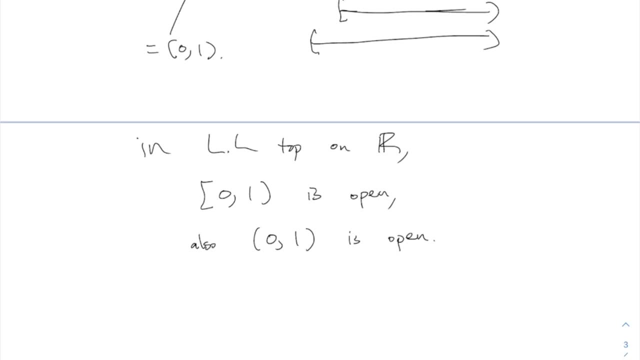 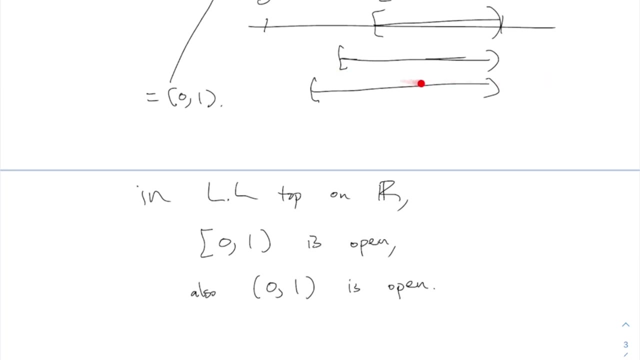 like is also a closed interval open, like one which has the bracket on both sides. can you make that by taking a union? you might feel like maybe I can do a similar trick of sets which grow to the right and take a union and get an interval which is includes both of its endpoints. actually, that is not. 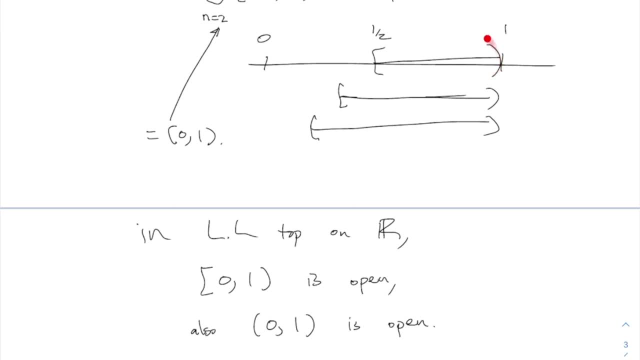 possible to do, although it's maybe not obvious, but since these sets all never include their rightmost endpoints, you cannot take a union of them. where the the right endpoints are, say, approaching some limit, you still don't get the point on the end, because none of the individual sets have the point on the. 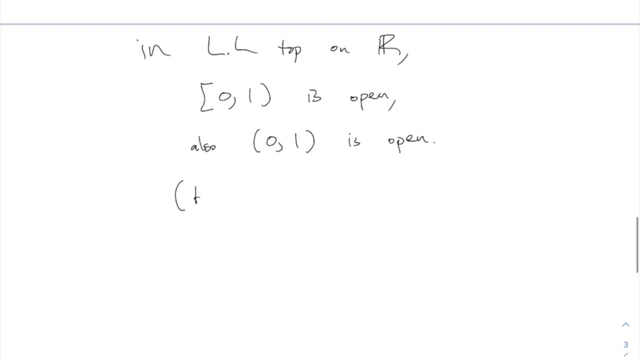 end. so actually, this is open, I will say. but something like this is not open. don't say closed, folks. you probably know by now closed is not the opposite of open. this is. this is a fact in real analysis. right, there's a closed just means something else. this is also not open. and also you cannot get a set like 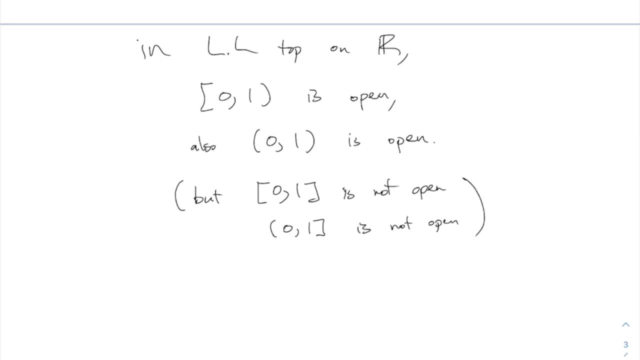 this. this is not open either in the lower limit topology- very weird. in my opinion it is intervals which are either open on both ends or include the left end point will be open sets in here, but not other types of intervals. all right, I want to talk about topologies on R2, but actually I have 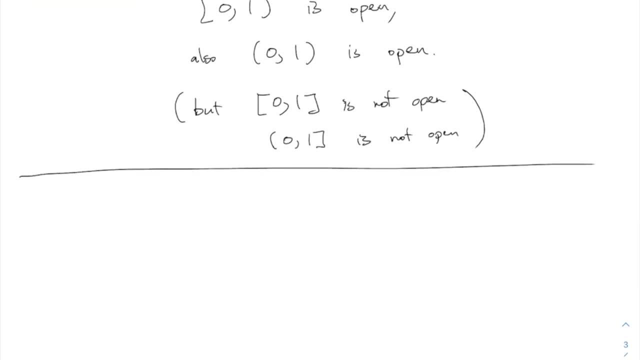 just one sort of random fact. I'm, you know, I am, I'm following along what they do in the book for the most part, and for some reason, the book throws in this random fact at the end of this little section here, which which is important, but I think it's important to know that. it's important to know that it's important. 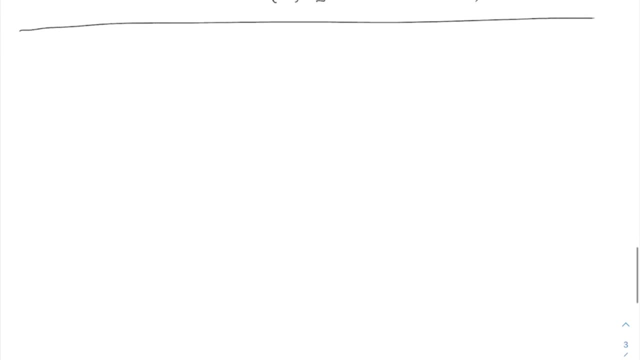 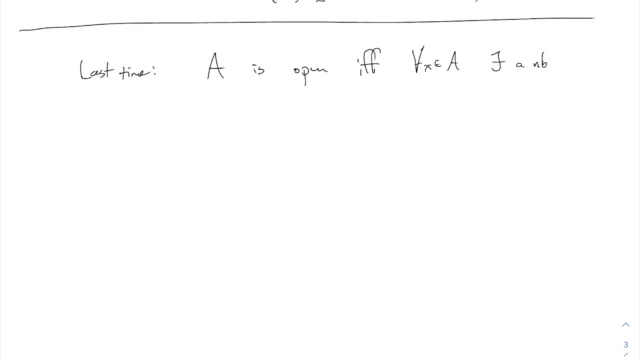 that says a is open if, and only if, for all X in a there exists a neighborhood you with X in you, which is a subset of a right. this is the code we have talked about. we have been doing this for a long time and we have characterization of an open set which is familiar from real analysis, that an open 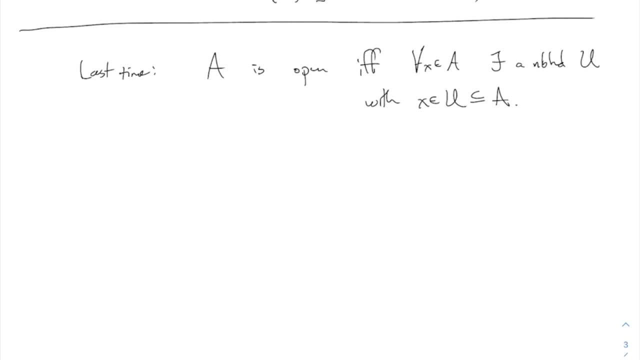 set. a set is open if, and only if, every point has a neighborhood around it. now, in real analysis, you you think of the neighborhood as being a very small epsilon neighborhood, but you remember generally, topologically speaking, the word neighborhood, it just means some open set which includes X, all right, so 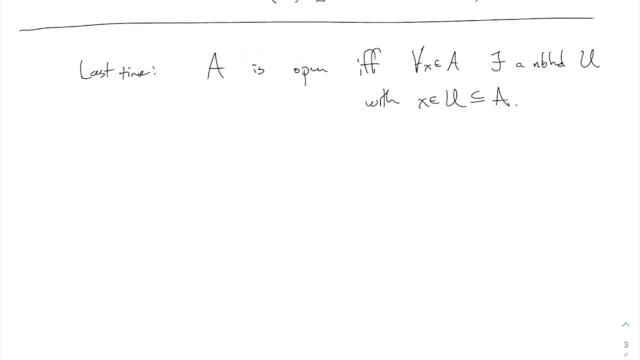 the whole set. a is open is the same as saying every point has a neighborhood which is contained in a. now, if you have a basis actually because of the intersections property, it means that if you ever have a neighborhood around something actually, you can shrink it down to a basis neighborhood. that's the. 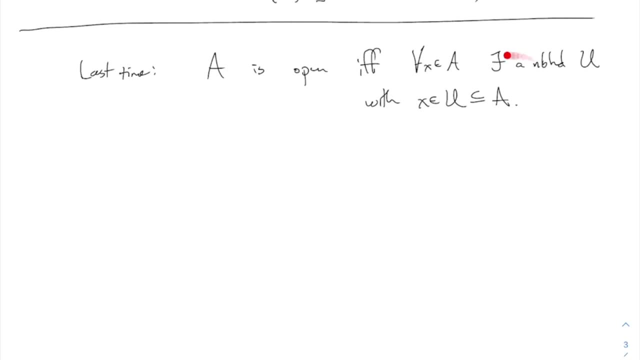 point of the shrinkable intersections property. so actually this you can say: actually, actually, actually- I wrote it, didn't, didn't look quite right as I was writing it. actually you can not only say that open means there is some neighborhood. actually, you can always shrink those neighborhoods down to basis. 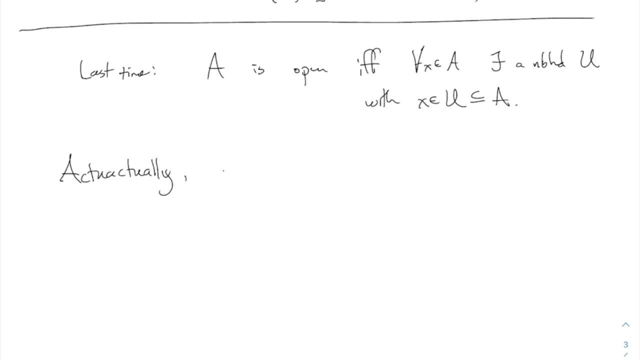 neighborhoods. so actually we can say stronger than that it is a fact. so I'll write this as a theorem. I don't want to go through the proof of this, but a is an open set. if, and only if, for all X in a there exists a basis neighborhood, I'll call it. 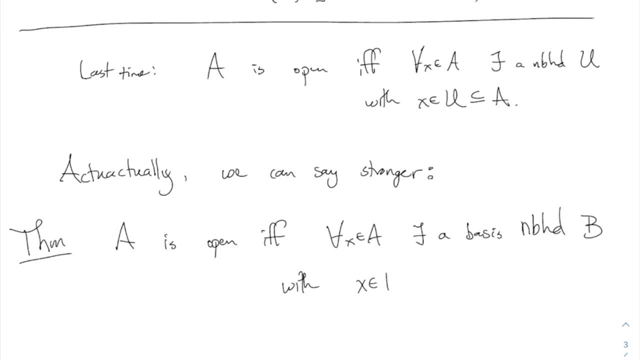 B, this time with X in B subset of a. all right, this will be useful sometimes. that an open set means you can always put a neighborhood around it, but that neighborhood it it doesn't have to be any old neighborhood. actually, you can. you can always make that neighborhood be one of your basis neighborhoods and 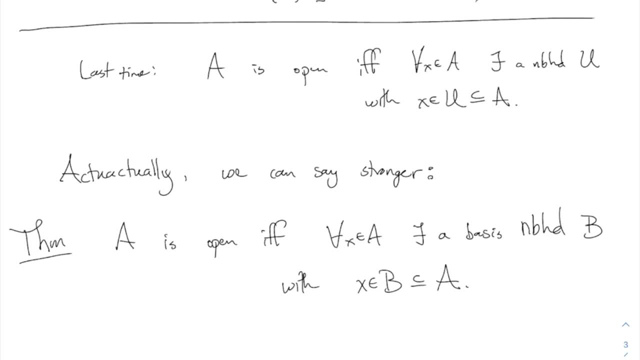 this is, of course, the way we always do it in real analysis, because we always take that neighbor to be some small Epsilon neighborhood and those are the basis neighborhoods in the standard topology. all right, this is just a. you can sort of file this away in useful facts, but we don't have a whole lot to 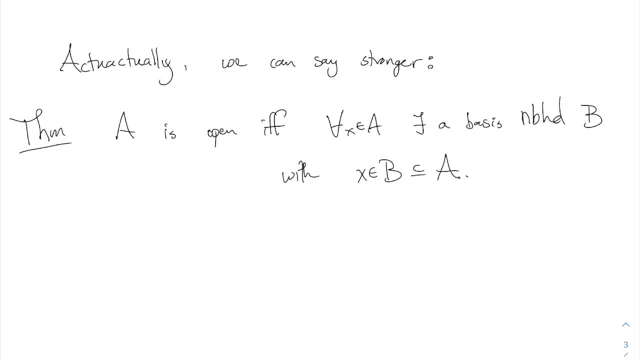 say about that right now. all right, great. I would like to talk about R2 then for a little bit, and, and actually RN for uh, for higher ends. I don't know if you were, um, if after, like the first day, my little introduction to the subject, maybe you're. 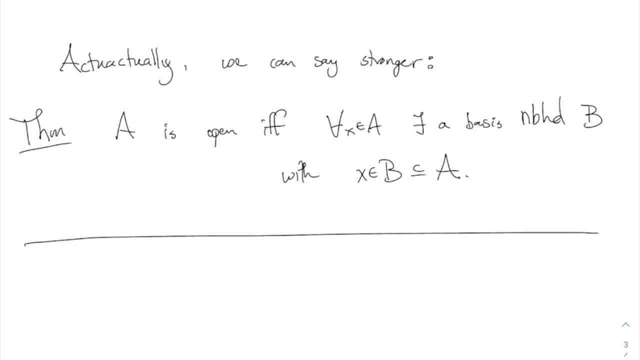 feeling really excited because you like you know drawing pictures and things a lot and you've been very, uh, disappointed by the class so far because it's just been a whole bunch of abstract nonsense. but, um, we're gonna actually like draw some interesting pictures. I mean, we have been 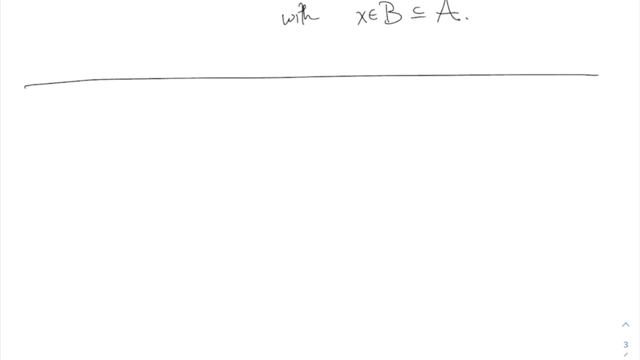 drawing some pictures. it's just that you can't really draw interesting pictures in R, which is basically what we've been talking about so far. R and also, uh, other abstract sets. that you all. But let's talk about topologies a little bit in R2.. Topologies in R2, can I just say, or Rn. 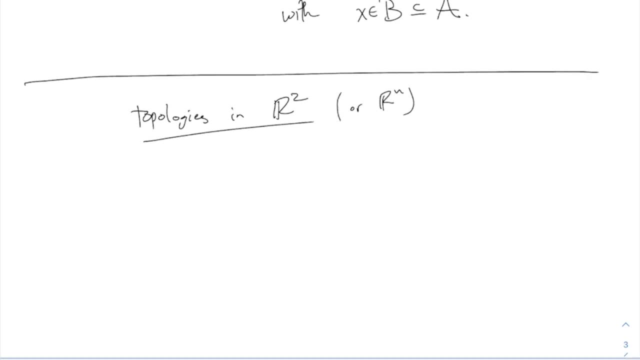 Really most of what we're going to say today about R2,. it works just the same in any Rn, but R2 is the easiest to draw the pictures. There is such a thing as the standard topology in R2, and it's the one which you get by using a certain basis. So to get the standard topology, 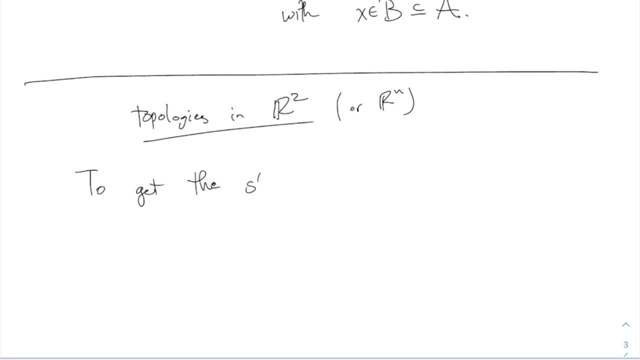 in R2, we need to decide on a good basis. That is to say, if you think of a point in R2, maybe I will poll the audience see what you feel we should do here. Here's some point X, When I ask you to make up a topology. 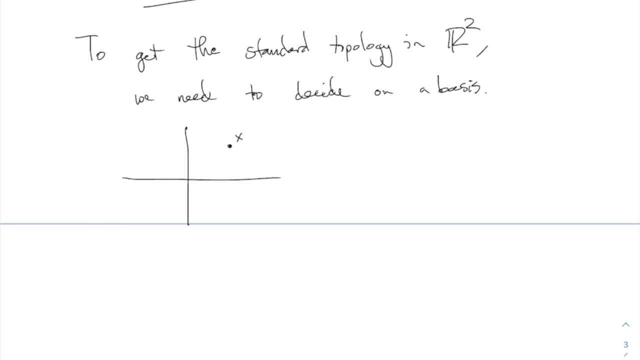 you can do this by deciding what your basis neighborhoods should be. Now, in ordinary R, the standard neighborhood of a point. this is my R2 picture, but remember in R1, in just R, the standard neighborhood that you always use is the epsilon neighborhood around X, which is sort of that little region of points. 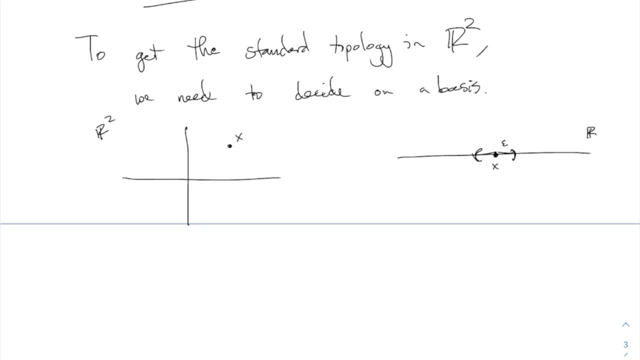 that are within distance epsilon of X and R. Anybody want to make a suggestion? What is the appropriate thing to do in R2?? I want it to be similar to that: All the points that are close to X within some distance. What would you say? 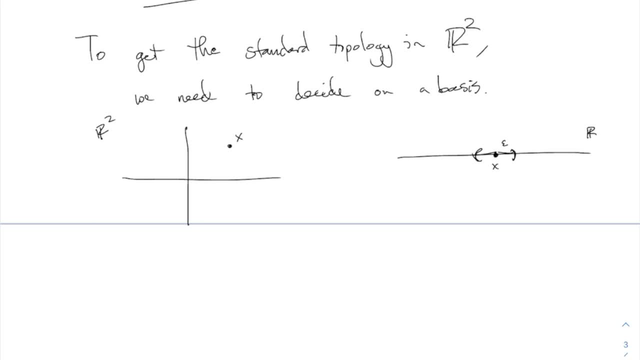 F, F, X, F, X, F. some distance. what would you say? Yeah, something like a circle around x. For the same reason as here, I'm not going to include the end points of this interval, So it's more like a circle. 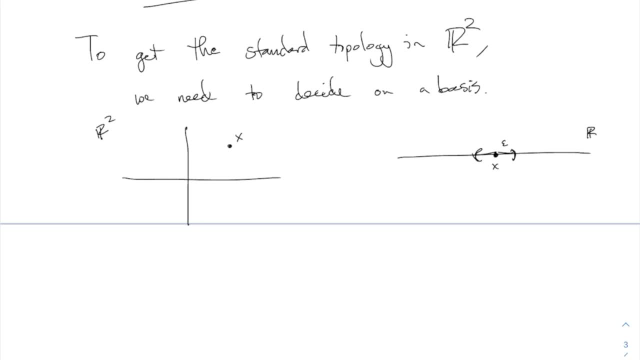 without its outer boundary. So I'm going to draw that like this. Sorry, I went right through the x, but this is that's meant to be a round circle with radius epsilon right. This is called the epsilon neighborhood around x in R2.. Actually. 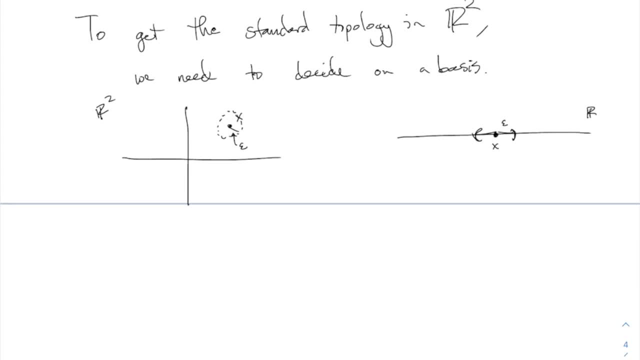 they don't call it in our book. they don't call it the epsilon neighborhood really, but this is called the open epsilon ball around x. all right, It is true, topologists talk all the time. It's often about balls, and all the bros can chuckle briefly about this. Get it out of your. 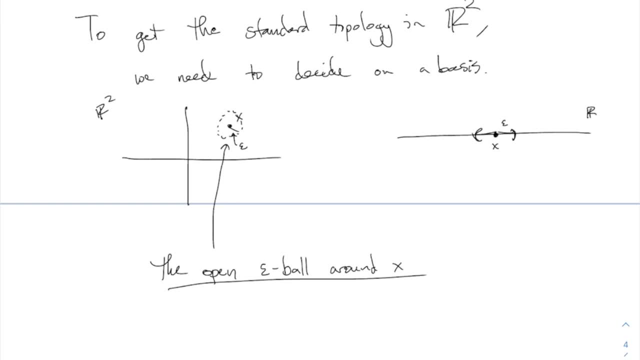 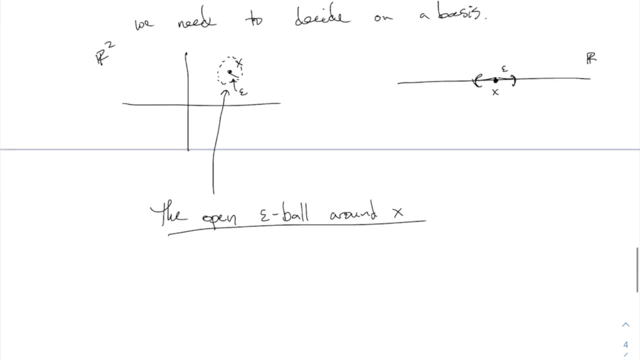 system, I am going to use the word ball. It's okay. The word ball means many things, including- well, actually, in my opinion, in R2, the word ball is not very appropriate for that shape. I would call this more like in R2, really it's like a disc. 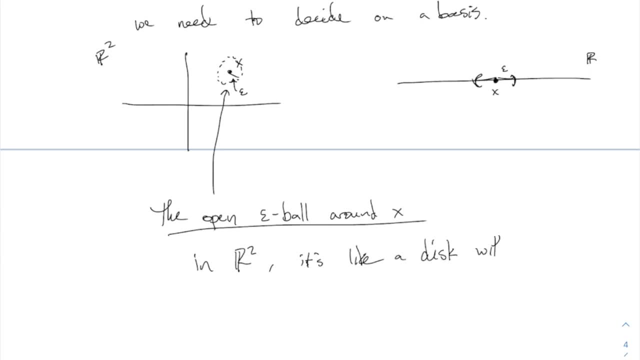 right, Without its boundary. But in R3, it looks like a ball that is the inside of a sphere without the boundary shell around the edge of it right, This is called the open epsilon ball around x. And in R2, it looks like a disc. In R3, it looks like a sphere In higher dimensions. it you know. 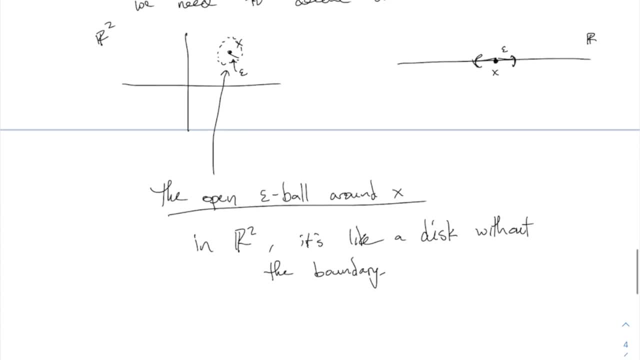 doesn't look like anything to me, but you can imagine it as being something like a ball in higher dimensions. all right, So the actual definition of this epsilon ball is the notation they use- is this: b of x comma. epsilon, That means the 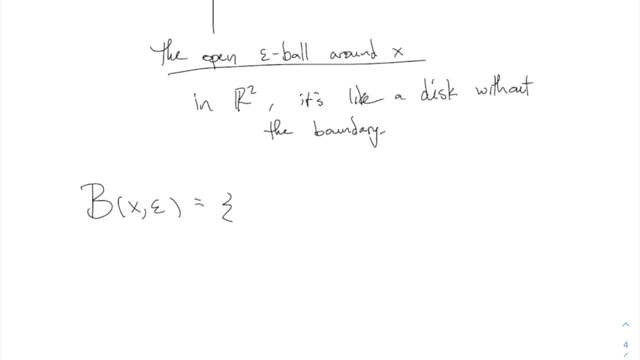 epsilon ball around x and the definition is: it's something like: it's all the points in Rn such that the distance from x to p is less than epsilon. All right, So you can do it in R2 or or any higher Rn's. This is all the points in Rn such that the distance 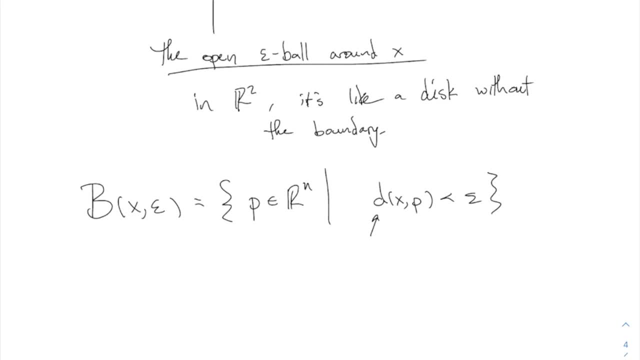 from x to p is less than epsilon, And this d is what they call the Euclidean distance. And just so that we all remember, how do you find the Euclidean distance? You do basically like a Pythagorean theorem: It involves a square root. 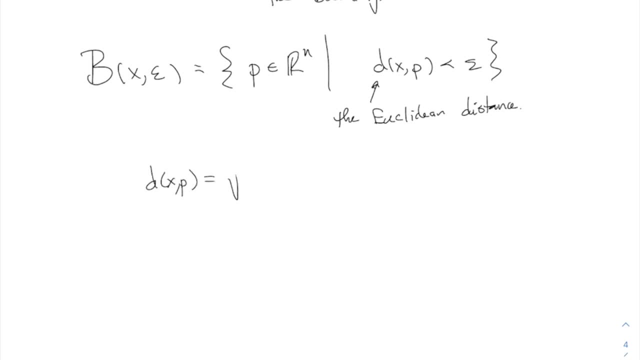 This is the formula for the Euclidean: distance is the square root of, and you subtract each of the coordinates. Sorry, I meant to write this. You have to write things in coordinates if you really want to find the distance. So if I write these as vectors, I'm talking about in Rn. 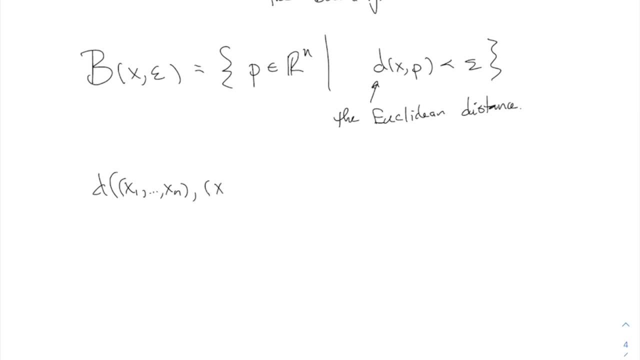 so it's like that The distance from x1 to xn to some other point, p1 up to pn- this distance is defined as the square root of x1 minus p1 squared, plus xn minus pn squared. This is the Euclidean distance function, which I am sure you're familiar with. 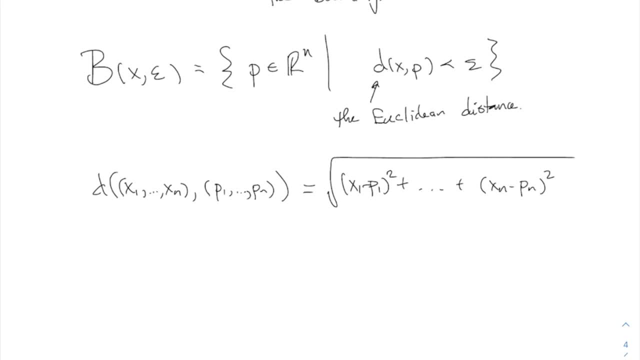 Not very, not very nice to use this formula to like actually compute distances by hand. It's a it's a pain to do, but we're not hardly ever going to actually do that. But we use it to define the. 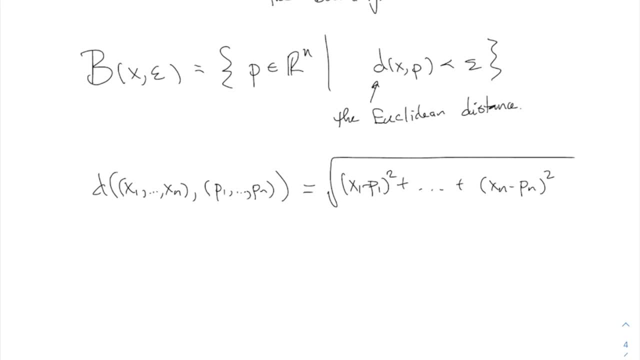 epsilon balls. All right, So let me just reiterate here: In R2, B of x, epsilon looks like a disk without boundary. In R3, it really looks like a ball, Again without its boundary. it looks like the inside of a ball. 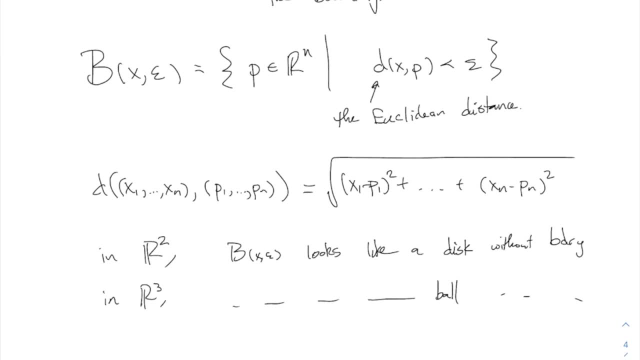 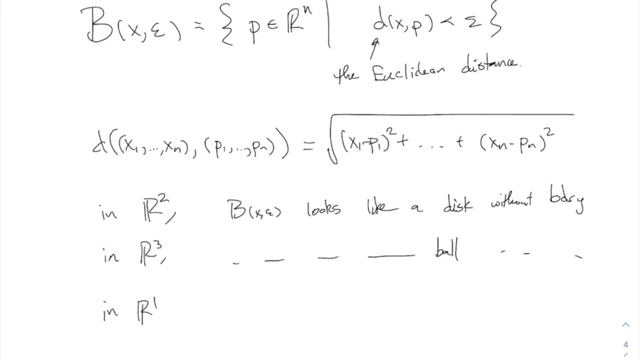 like the solid part- Okay, a ball- and in higher dimensions it's i. i don't think of it as looking like anything, but it's like a higher dimensional version of a of a solid ball, and actually the same formula you can use in r1. what does that look like in r1? this would be all of the other, i guess, if x is just a single. 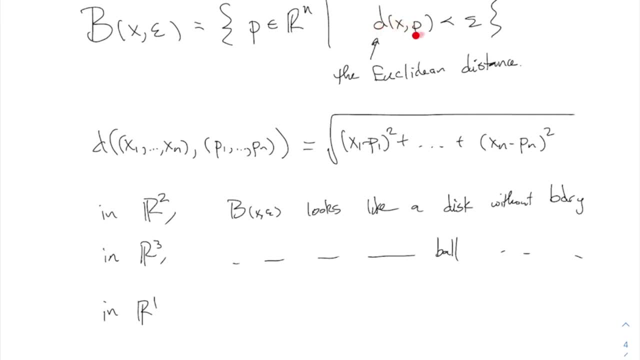 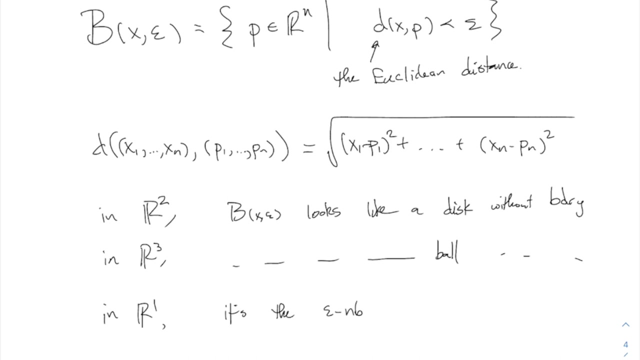 number and p is some other number that just says the. the distance from x to p is less than epsilon. actually, that is the same as this little interval, right? it's this the same definition. so in r1 it's the- uh, epsilon neighborhood of x, right? so actually this ball is, strictly speaking, a. 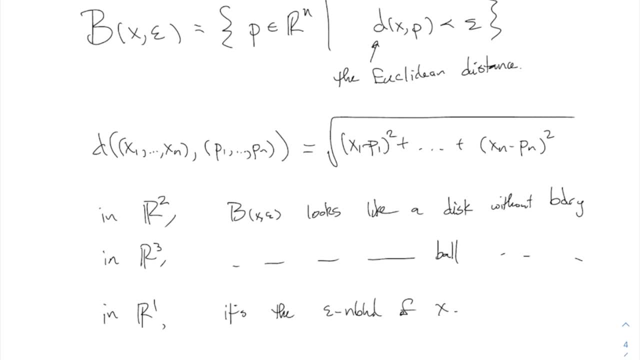 generalization of the one-dimensional epsilon neighborhood. it's what you get when you try to do the same thing, but in higher dimensions you get a circle, a circular like thing or a solid ball like thing. all right, all right. all right, we should at least briefly discuss. 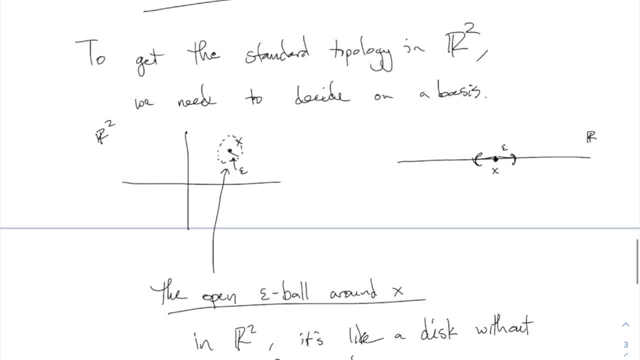 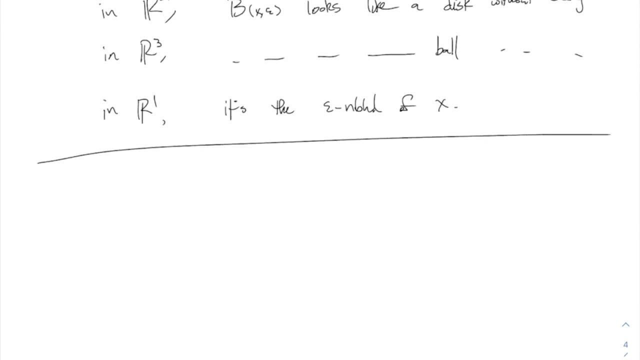 why this makes a basis all right. so we need to decide on a basis. we're going to use sets like that for our basis, so the standard basis that we use- um, let's just talk about this in r2, just because i'm going to draw some pictures and it'll look nicer there. but in r2 we can use 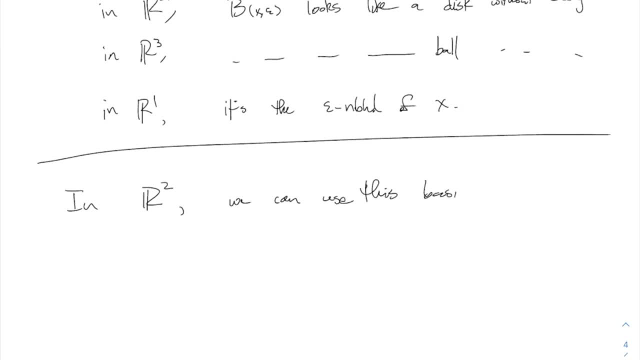 this basis. b is the set of all things that are, you know, epsilon balls, such that x is in r2 and epsilon is some real number greater than zero. all right, this is what we're going to use as our basis, and the topology it generates is called the standard topology on r2. 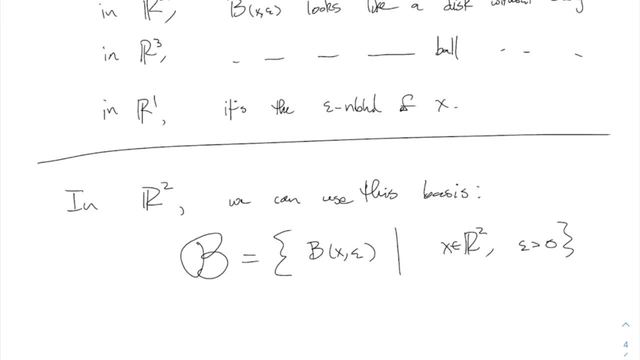 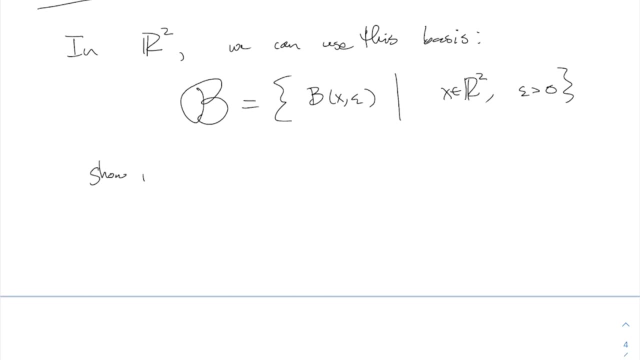 we should convince ourselves again that this really is a basis. let's show it's really a basis. remember. you must demonstrate the two properties right and remember what the first property was of being a basis. it's the easier one. the second one is the weird thing about intersections, but the the first one is: 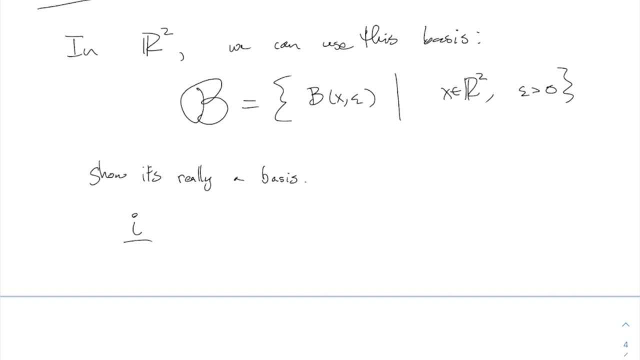 yeah, yeah, we have to show that these balls cover all of r2, that is to say, every point in r2 is actually in one of these balls. but that's, that's definitely true, right, but anyway, that's what we have to demonstrate. so i'm going to say: uh, this is like just to refresh our memory, this is the covering. 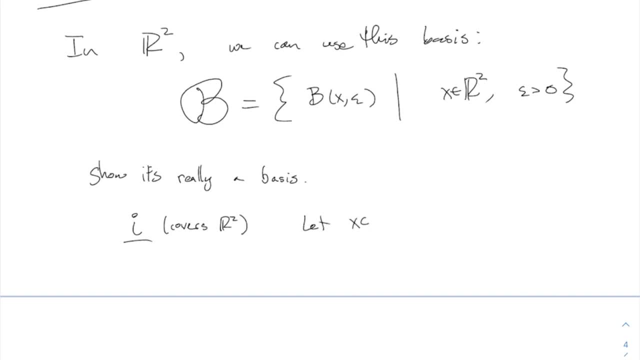 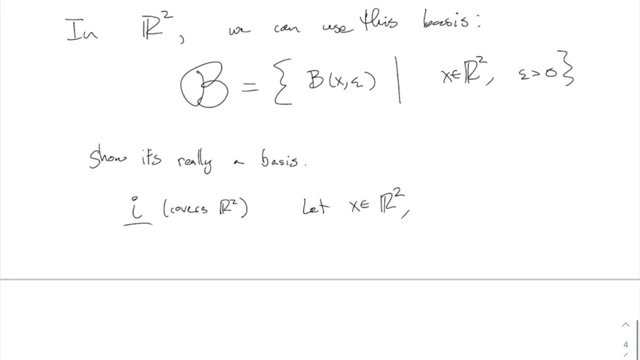 property. so i say something like: let x be in r2. really everything i say here works in rn, but uh, let x be in r2. then x is an element of. can somebody tell me like it has to be? uh, it is an element of the ball around. 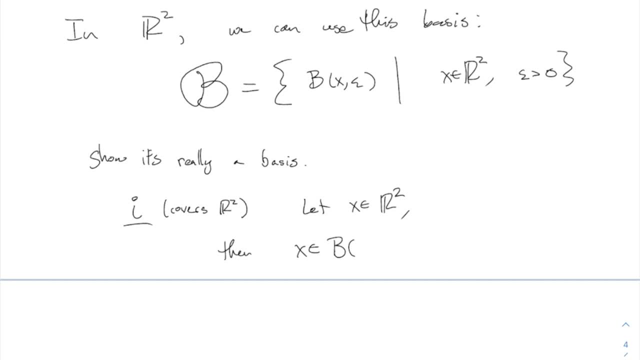 you should tell me: uh, what's the center point of this ball and what's the radius? anybody any thoughts? if i show you a point here x, is there actually a ball which includes that point? yeah, can you show me a point here x? is there actually a ball which includes that point? 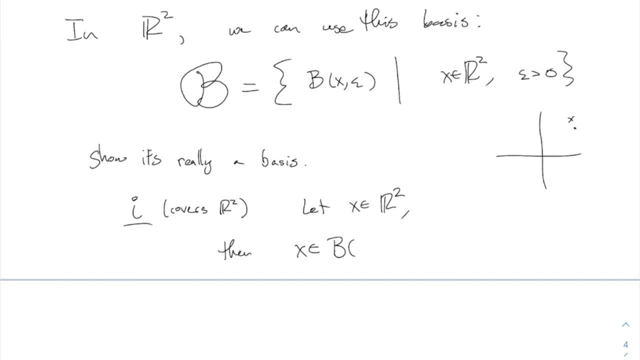 can you tell me like, can you say, yeah, center that x and the radius is? you should say a specific radius. there are almost no wrong answers. one, yes, that is the correct answer, is one, although you could have said any number here greater than zero. but uh, yeah, x is always inside the uh ball centered. 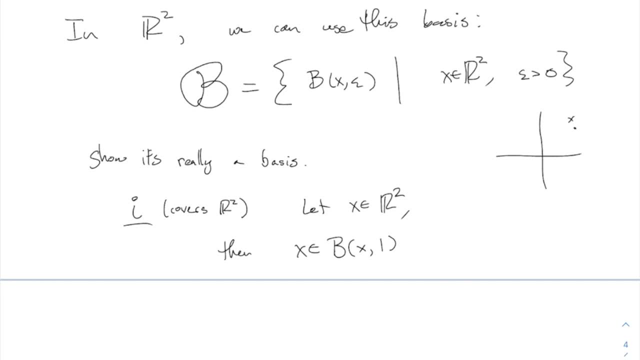 around x of radius. whatever one is the most sensible thing to say here, but you could have said anything, all right, okay, that's it. so every point is actually part of one of one of the basis balls. and the second property. this is the intersections property. this is the. 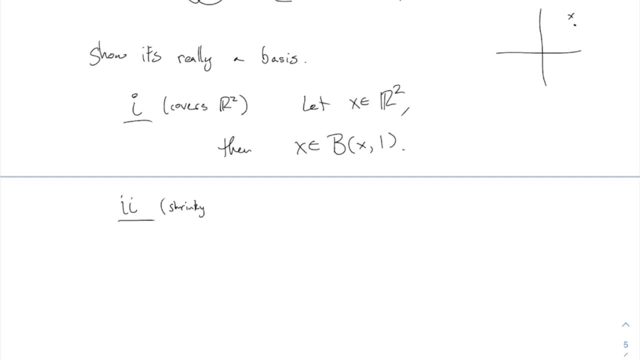 shrinky, shrinky property. um, that says, if you have a point which is in the intersection of two balls, so there's a. this is the same picture that i usually draw, but actually this is i suppose i should. i should use this dotted line. so here's, here's one ball, i'll call that b1 and then another. 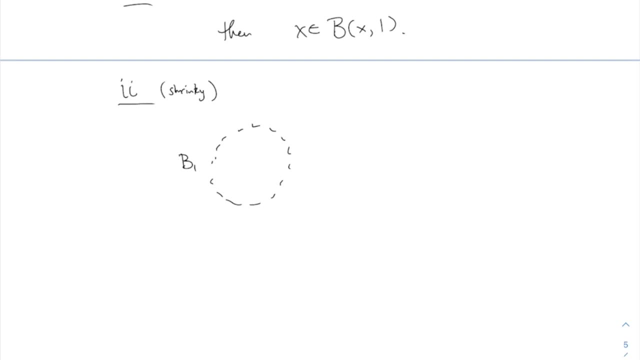 ball and they intersect. now i'm going to try and draw them so that they they may have different center points, they also may have different radii radiuses. so something like i'm going to make it, i'll make it bigger. how about? i'll make this one giant? 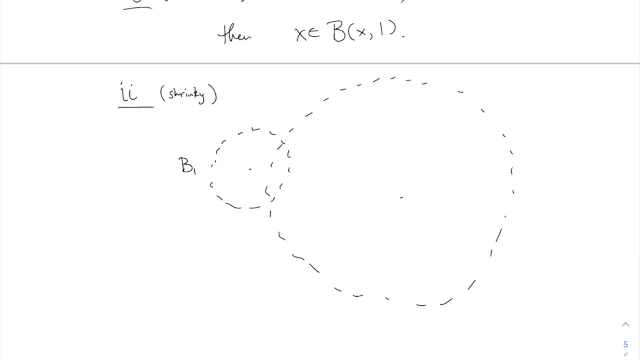 here are two different, uh, epsilon balls which have some intersection, and let's imagine that i have some point in the middle x. i don't want to write out a detailed proof of this, but is it true that there's actually a ball around x inside the inner? the overlap? yeah, there is. i mean you would. you might have to choose the radius. 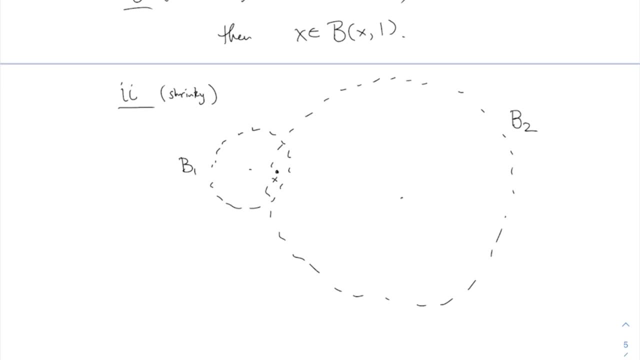 to be very small, but there there definitely is a ball around x. so in this situation, i would just say, if b1 intersect b, if x is in b1, b2 and those are two big balls, there is a little ball. inside the intersection around x there is some uh b3, which will be the ball centered around x. 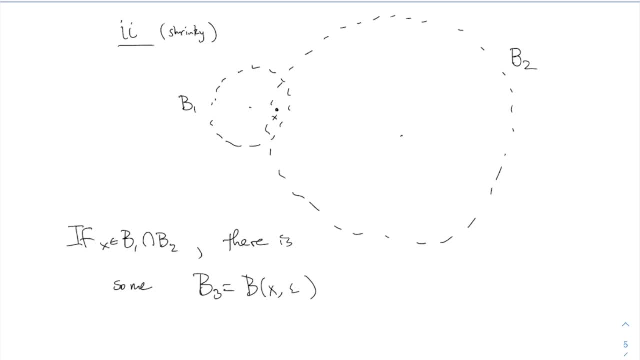 of radius epsilon. now it's actually slightly complicated to say what epsilon should be. you might feel like if i know the two radii here, then i can choose that epsilon to be like the, the minimum of two radii, the, whichever one is smaller. but actually that's not small enough because in this case 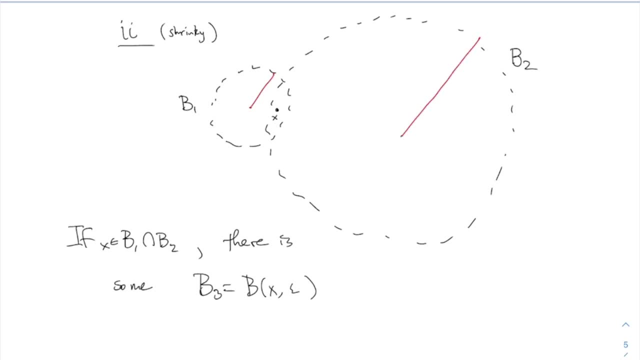 this radius? i have two radii right, but the the radius required for this little ball is much smaller than either of those two. now it is, it is possible to work out the details and sort of give give me a formula for how small exactly this epsilon has to be in terms of these other ones. 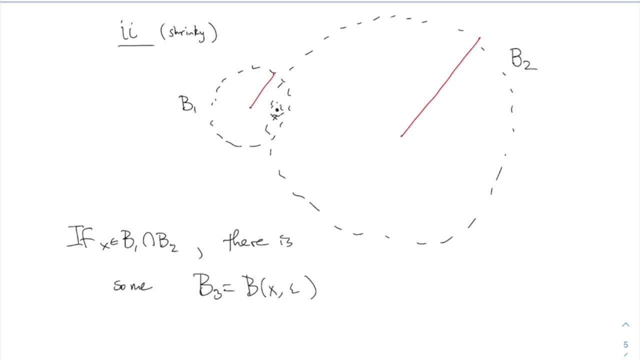 but i don't really want to get into the details of that. it has to do with what these two radii are and then also how far apart the two centers are. you can do some kind of triangle inequality type thing. the details of this are in the book, but i find them. 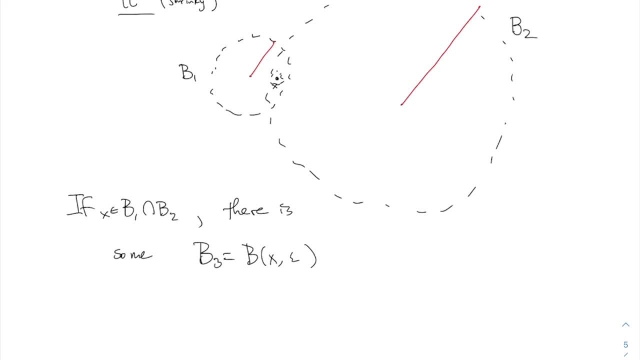 somewhat uninspiring for what is really an obvious fact. there is a little ball around x, which is inside the intersection, so there is some ball around x of radius epsilon, with ball three is in the intersection and of course, x. x is in there. all right, that's the intersection's property, to demonstrate that it is a basis, all right. 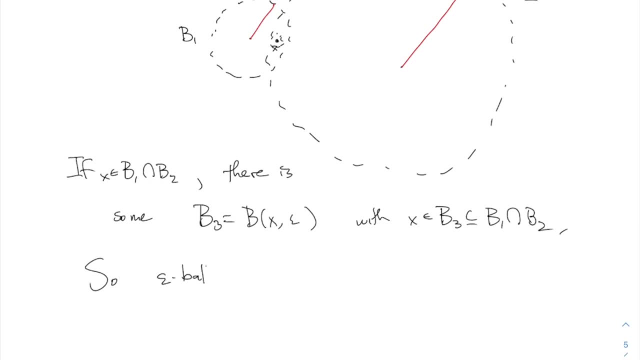 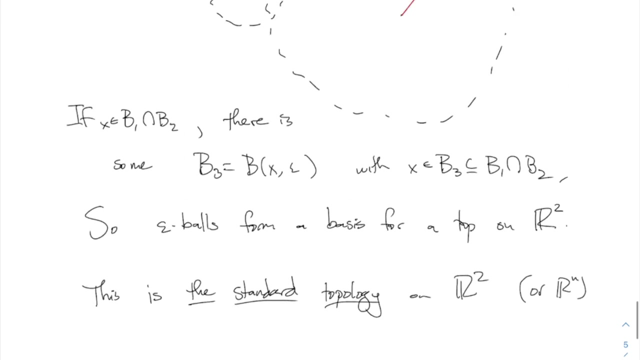 so i will just say the epsilon balls form a basis for a topology on r2 and that topology is called the standard topology on r2. so this is the definition of the standard topology on r2. can i just say parenthetically: or rn, you just do the same thing. it is also true, the only. 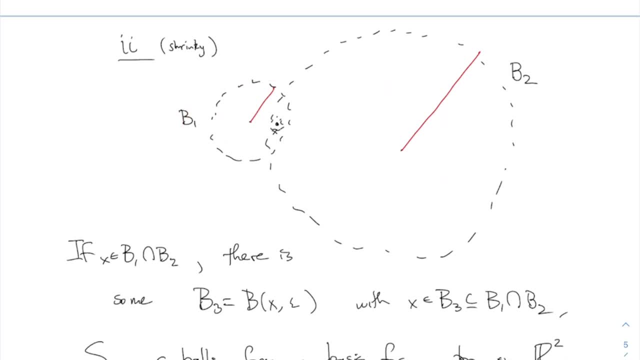 thing that you need to be concerned about is this same thing true in higher dimensions? if i have, say, two three-dimensional balls and they have some overlap, can you put a tiny little three-dimensional ball inside the overlap? the answer is yes, you can so, and it works in even. 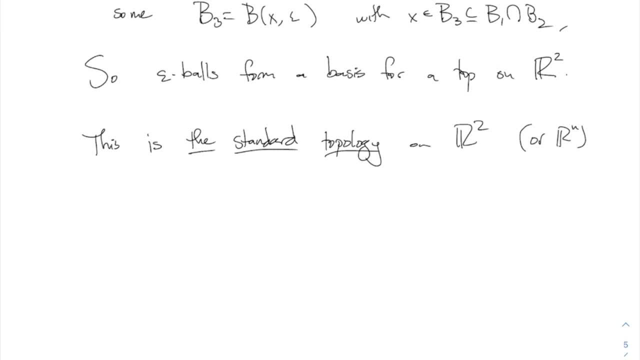 higher dimensions than three. all right, this is called the standard topology. on r2, it is generated by a set of balls. so, uh, an open set in r2 is any set which is a union, perhaps infinite union- of, uh, of balls. all right, uh, you might wonder, does that mean that open sets have to be sort of 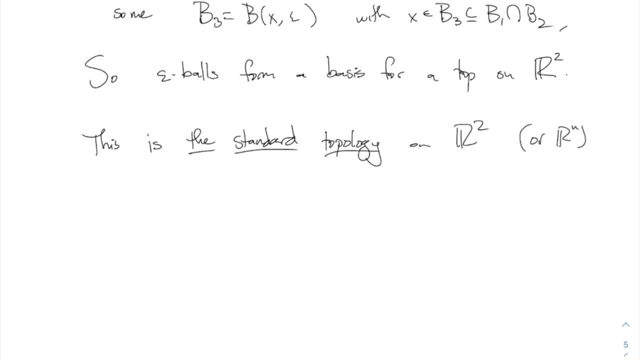 ball shaped. if it comes from, it has to come from taking a union of of balls. does that mean that it has to look like a um, like it has to have round edges to it or something like that? that's actually not the case in uh, in the standard topology on r2. so 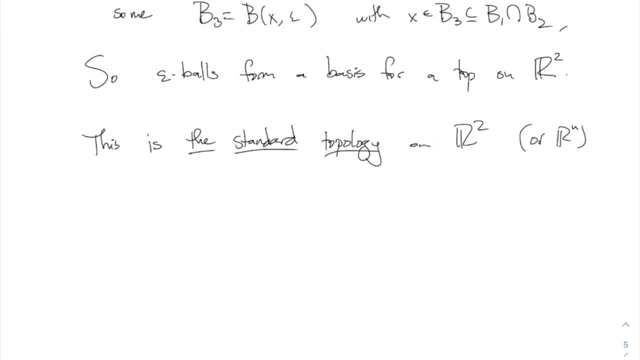 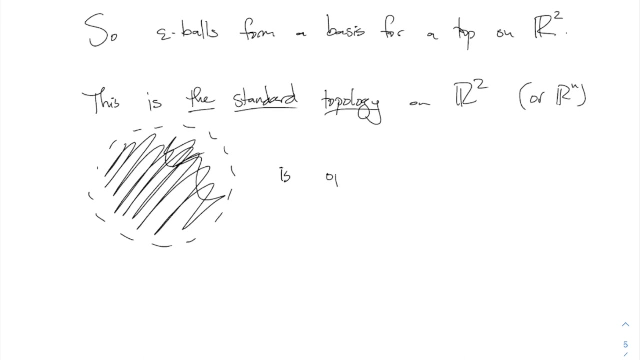 can we? i'm just going to draw a bunch of pictures here. um, how about i draw a set and you say if it's open or not? so the standard example is, you know this, including of course, all the points on the inside, but not the boundary. this is open, obviously, because that is one of the uh open. 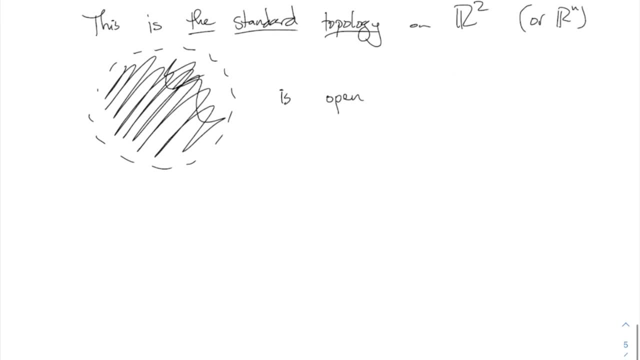 balls, so that one by itself is definitely open. what if, though, i had a set which was sort of: um, how about this? a triangle like that, including all of the interior points, is that open? can you somehow? the question is, can you represent this as some kind of union of open balls? now you might feel like 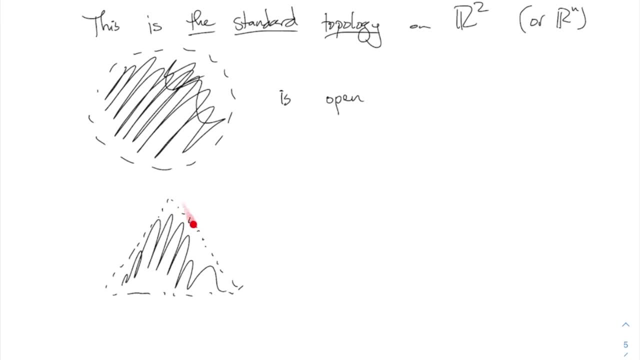 i don't know. to me it feels kind of like that's not going to be possible to make this straight edge out of a bunch of individual balls as a union. that doesn't seem like it's going to work out. but actually it's not so clear because we can use infinite unions and infinite unions. 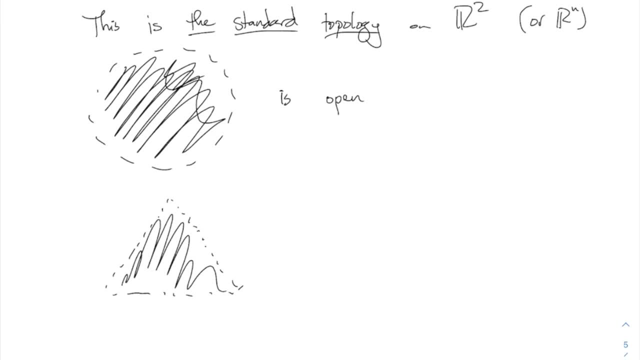 do weird stuff, like you saw in the lower limit example. you can take an infinite union of lower limit intervals and get an open interval, which is very weird. you can take an infinite union of ball like shapes, and maybe they end up being a straight edged shape. actually, this one is also open. it's better, in fact, not to think of this, as 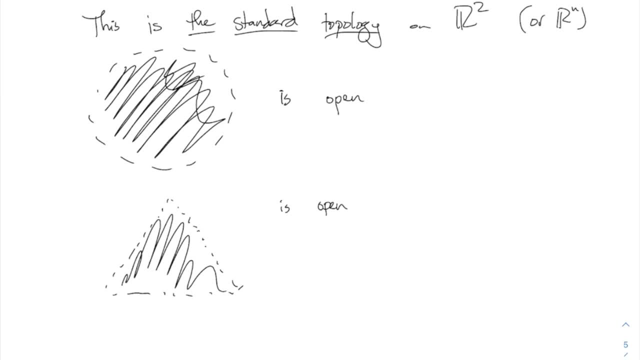 can i make this? by a union of balls? it turns out you can, although it's very difficult to see that that's really true. really, all that matters in deciding whether a set is open or not, think of this in terms of neighborhoods of a point. if i choose any point inside this set, let's say x, right? 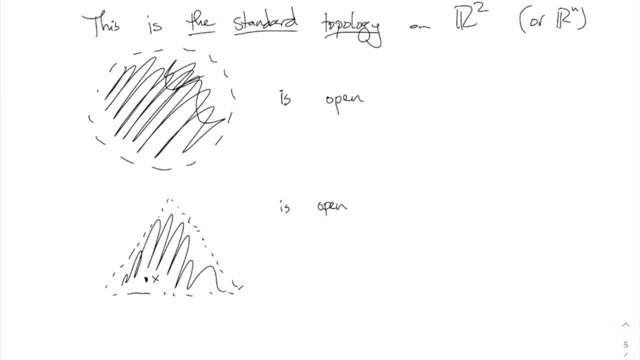 here. does it have a neighborhood around it which is still inside the set? yeah, it does. that means it's an open set, right? because because of that theorem that we just said, an open set means that every point inside the set has a neighborhood which is contained inside the. 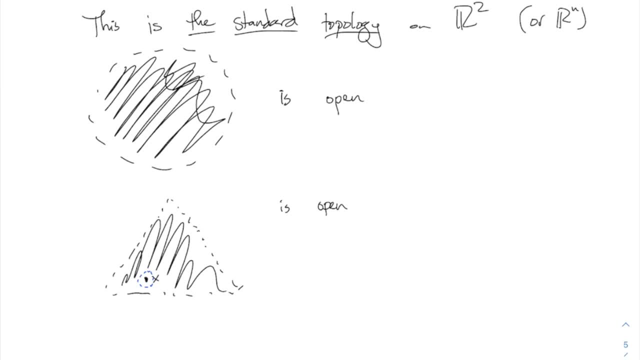 set. so this point here: it does have a little ball around it which is contained inside the set and you can do that for any point in your set. this is why it's important that the boundary is not included. right, you did include the boundary, then your neighborhood would stretch out outside of the 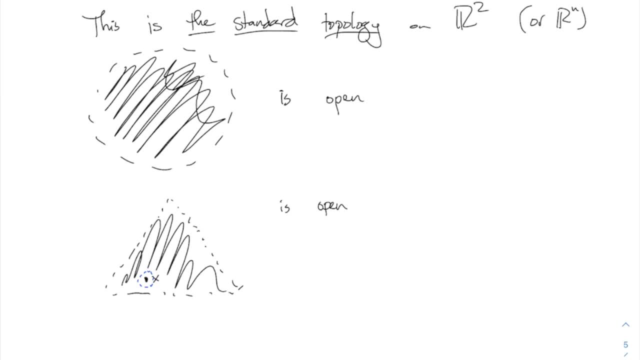 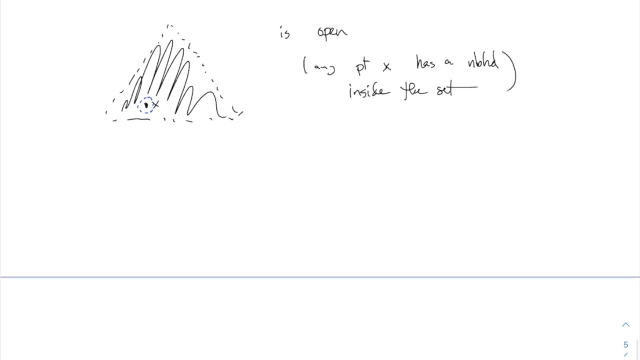 set. but anyway, this is open the uh. it's not easy to express that as a union of balls, but it is easy enough to see that any point x has a neighborhood inside the set. this is sometimes a more appropriate way of thinking about it. all right, uh, how about something like? here's a more interesting one. 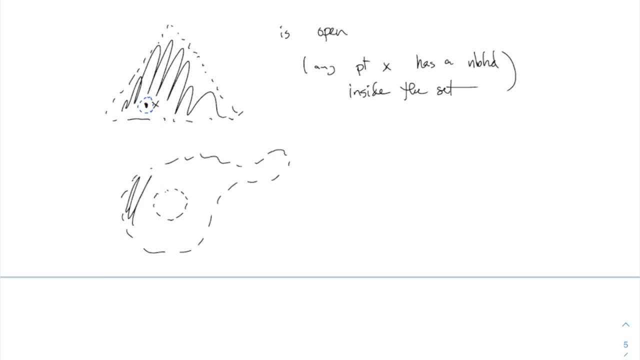 here's a weird looking sort of blobby set with a hole inside. is that an open set? you should again be thinking about if i, if i choose any point in there, can i put a little ball around it, which is still inside the set. you want to show me the thumbs? yeah, you think. is it open or not? people are looking around at the. 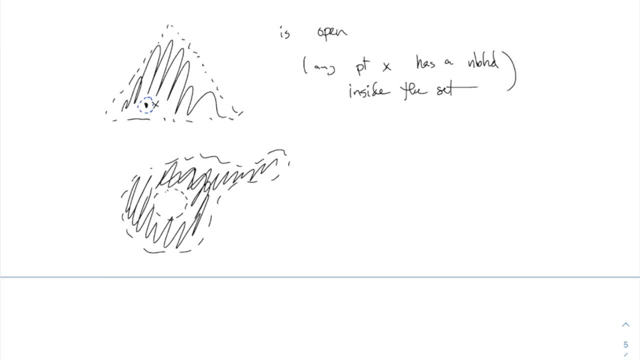 others though thumbs before committing. you got to commit to the thumbs. the thumb should be up. yeah, this is an open set. if you choose any point in there, i don't know say like, right here, can i put a little ball around that which is still inside the set? yeah, you can, even if it's really close to the edge. 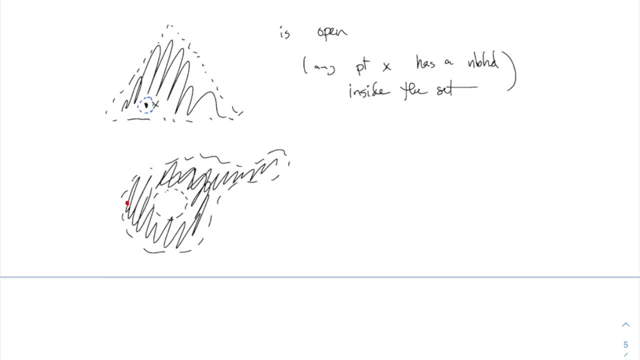 you can make a really small ball which still fits inside the set if it's right on the edge. you can't do that, but this set does not include the points that are right on the edge, so you don't have to worry about that. so this one again is open. all right, uh, how about? 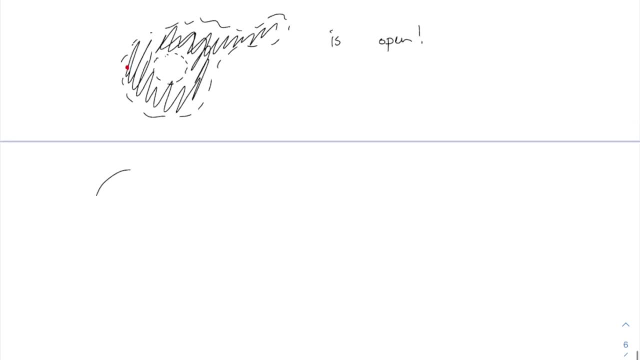 here's an example of one which is not open: something like a circle which includes the boundary. all right, this is not open because i could choose a point right on the edge, and now that point does not have a ball around it, which is contained inside the set. 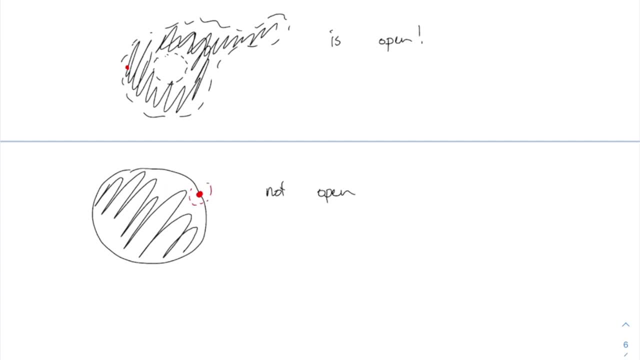 because any ball around that point will automatically stretch outside the set a little bit, and so it has no neighborhood. that's contained inside the set, so not open. this is because the boundary points have no balls inside the set. any ball around one of those boundary points will stretch outside and that means that it is not an 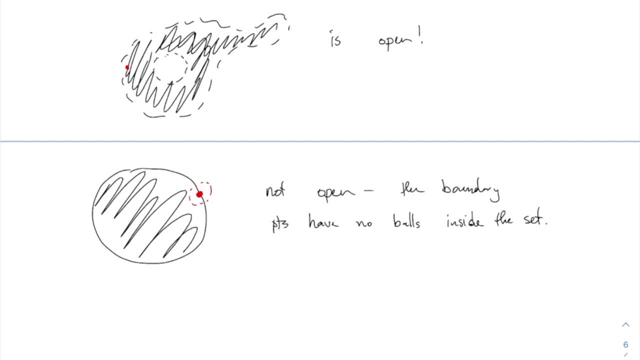 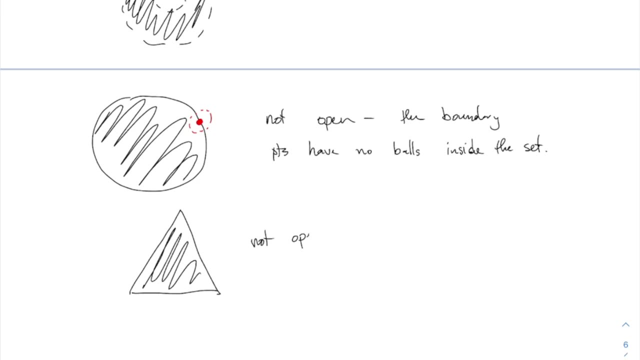 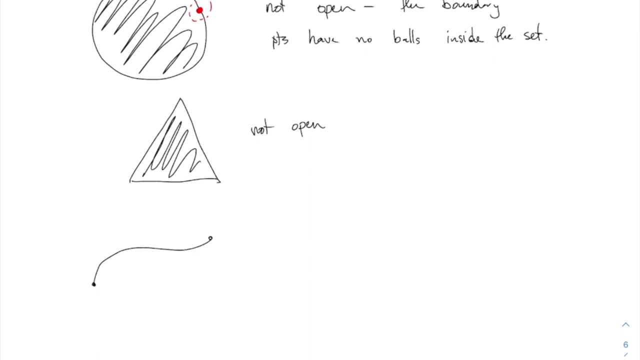 open set, all right. uh, how about you know similarly some something like this: a triangle with its boundary- this is not open for the same reason. or, uh, a set which is like in r2. you could just do something like that. right, that's a, that's a subset of r2 which looks like a curve, a parameterized curve, or the. 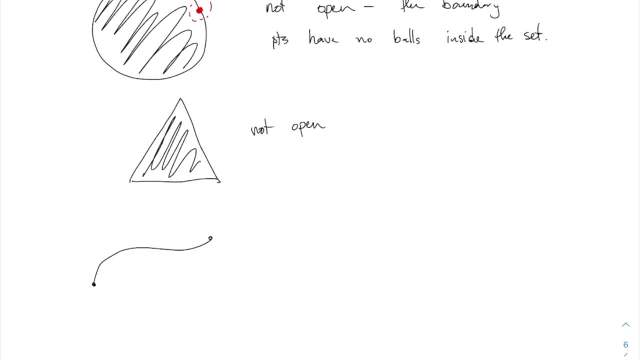 graph of a function or something. is that open? what do you say? yes or no? the question is still: can you put a ball around each one of those points so that the entire ball is part of that set? no, because that that set is only that curve right. so again, you could say: choose this point, any ball. 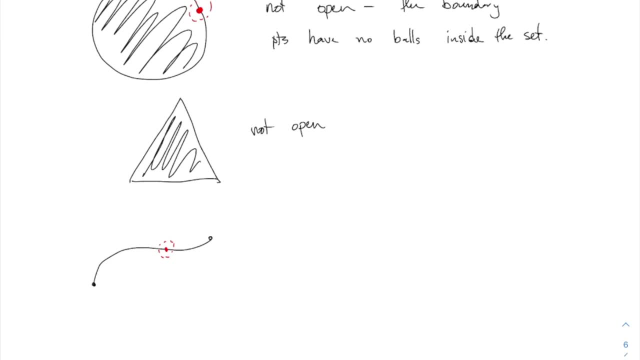 around that point automatically stretches outside that curve. so this is also not open, all right, or we could talk about even weirder shapes that you can't really draw, like how about um? how about q? you ever heard of q2? q is the rational numbers, q2 is just points are reversed. 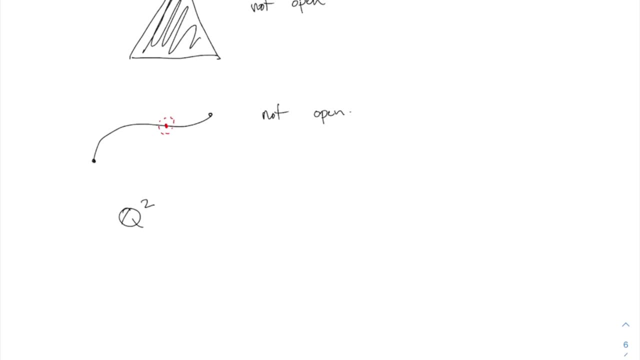 in R2, having both coordinates being rational right. This is a subset of R2.. You can't really draw a picture of it. It looks like some kind of cloud of points which exists everywhere. It's dense in all of R2, just the same way that Q is dense in R. 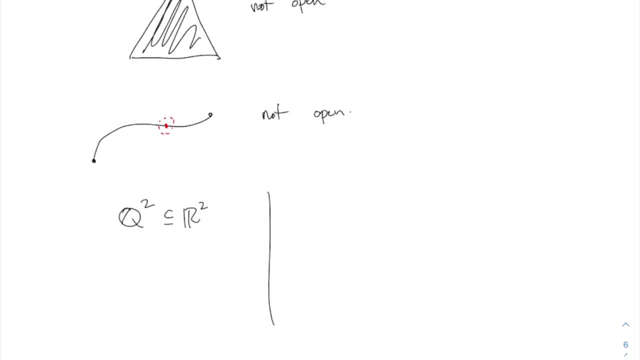 Is that an open set? So I think I imagine this set as being sort of it's everywhere, but it's only the points which are rational values, And you have to ask yourself if I choose some point here with two rational coordinates. is it true that all the points in 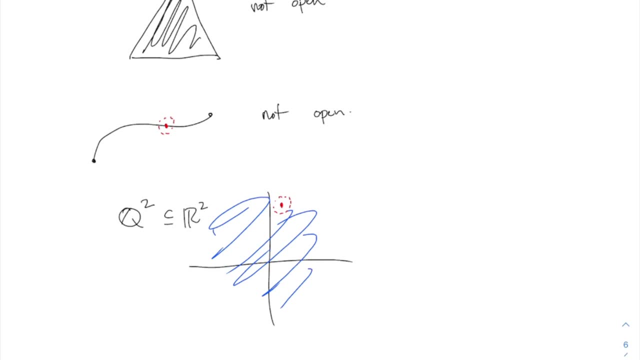 the ball around it also have two rational coordinates? The answer is no, they don't. You're going to have some irrational coordinates in that ball because the ball includes all real coordinates within that distance, not just the rational ones. So here, not open. This Q2 is not. 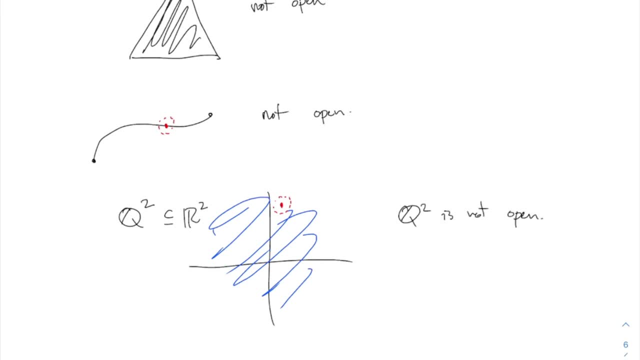 open, All right, Just like Q. ordinary Q is not an open set inside. If you take a neighborhood around a point, it's not all going to be rational values inside that neighborhood, All right. One more thing to say about this. We got a few minutes left here. 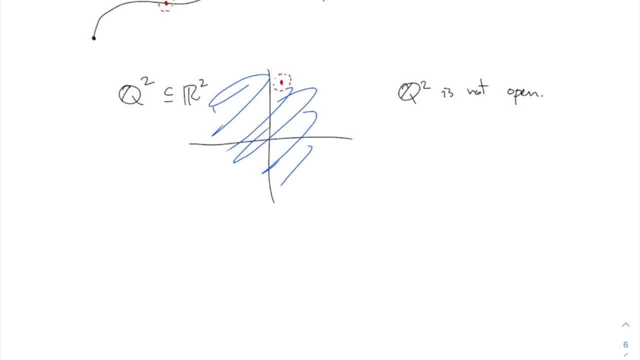 All along we have been using the balls as our basic neighborhoods in R2.. And it was Alvin's idea to use the balls right Now. I predicted that at least one of you would have this idea, But I don't think so, So I'm going to go ahead and do that. 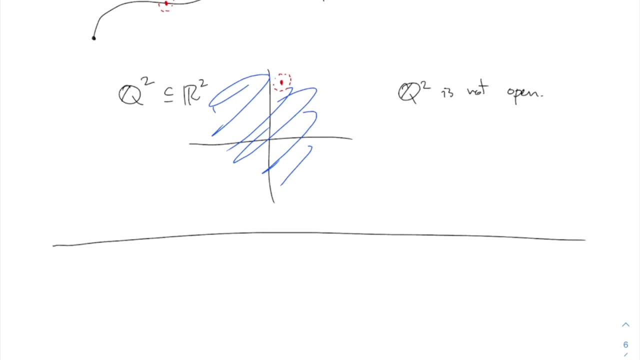 Which is why I prepared all of this business here. But I don't know if anybody was thinking: did it have to be balls? Did anybody have another idea when I said: what should we use for the neighborhood around a point like this? I don't know. Did anybody- Here's another idea? How about? 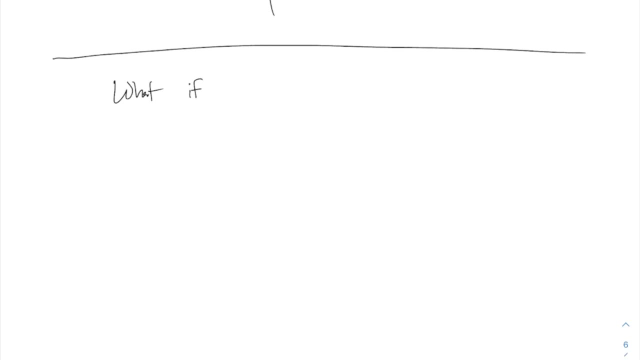 what if, instead- and I'm not going to give you some ridiculous other idea- This is a totally reasonable thing- What if, instead, we used boxes like this, Like a square box- I don't care if it's a square, exactly, but a rectangular. 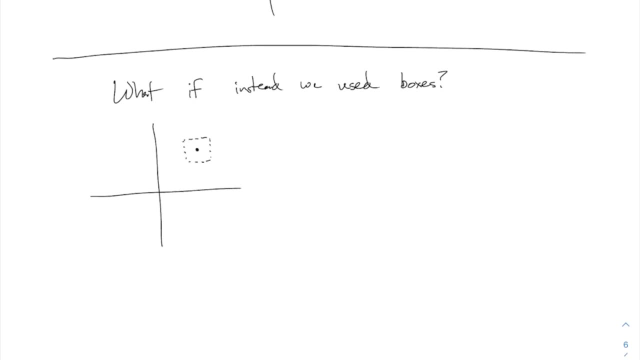 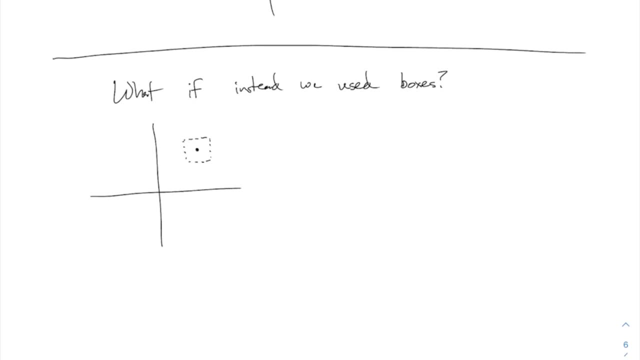 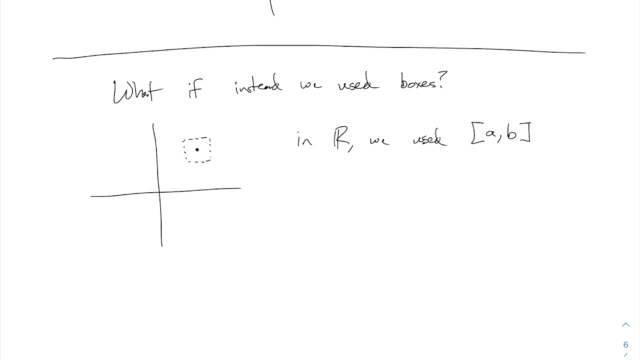 two-dimensional version of an interval. When I think of a two-dimensional version of an interval, I think of a little square right. It's an interval on one axis and an interval on the other axis. That's a two-dimensional interval. So in R2, then maybe 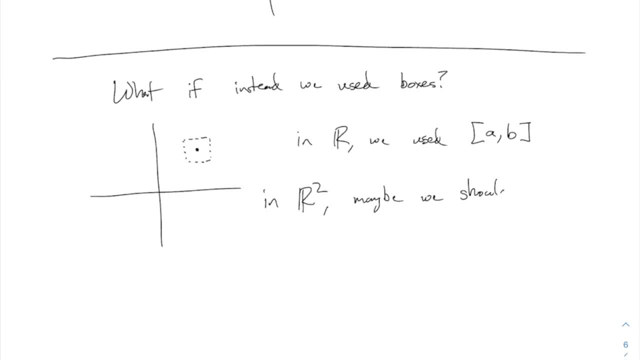 we should use something that looks like A, B, cross, C, D. This would be the product of two intervals And that looks like this: right, Sorry, I'm writing closed interval. I should have been writing open intervals this whole time. Sorry about that, Of course we don't. 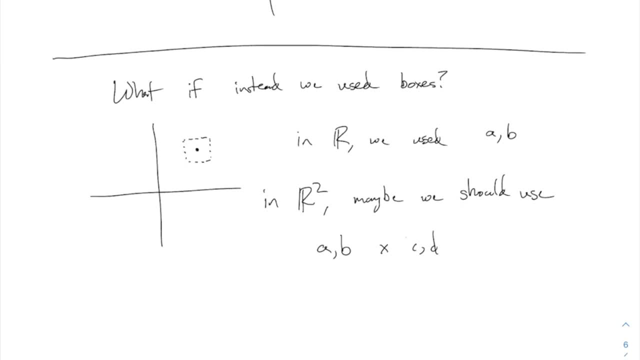 include the endpoints. If you decide to include some, or you know all or some of the endpoints, then you get some weird things. There is such a thing as like a lower limit topology on R2, but I'm not trying to talk about that, at least not at this point. 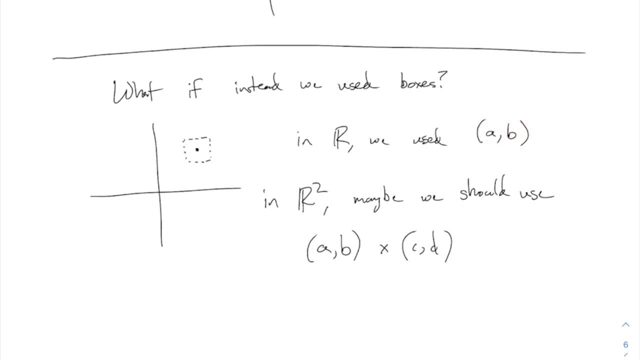 Anyway, in R we use open intervals like this. I think in a certain sense it is more natural, rather than using those circular things. it's more natural to use sets like this And, in fact, if you actually want to do computations, this is much more convenient. just because the Euclidean 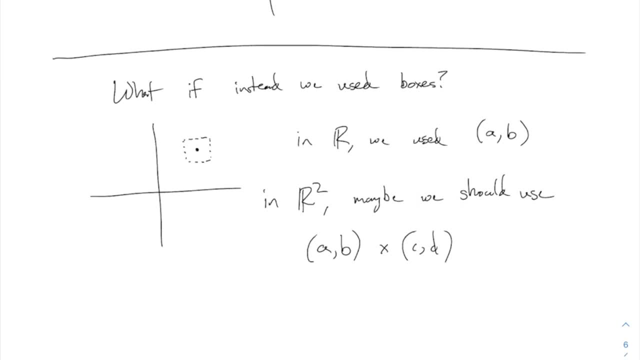 distance formula is a real pain to work with because it has the square root and all that business, Whereas this is a much more easy set to work with if you really care about doing a lot of details of these things. So my question is: is this a valid approach And if so, what? 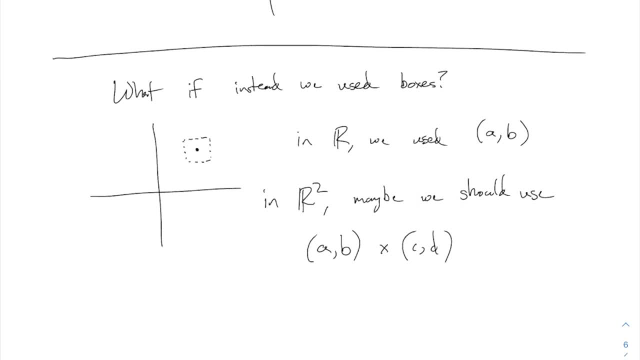 happens in terms of the topology that you get on R2 using these things. instead, The first thing we should think about is: does this still make a legal basis? So maybe this isn't even a basis, which is why we went with balls rather than boxes, But actually this is. 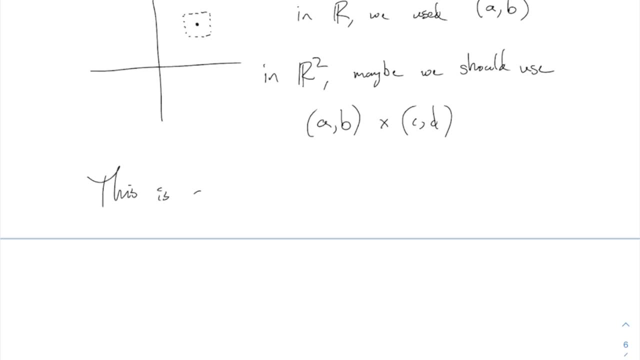 still a basis, And if you look at R2, you'll see that R2 is a valid approach. And if you don't really understand R2, you're gonna be pretty surprised by things like this, because the R2 number is a valid approach. Okay So, 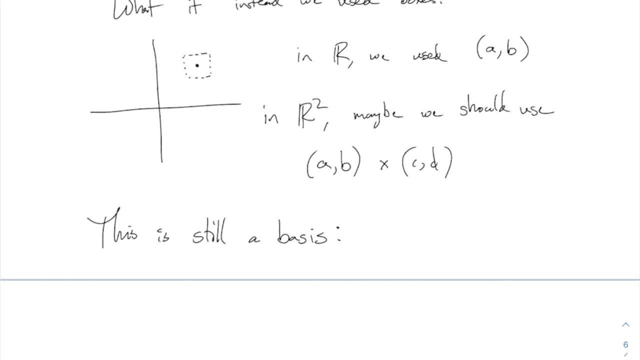 I don't wanna go through all of the details, but first of all I hope you see that every point in R2 is contained in one of these boxes, So the boxes do cover all of R2.. And then also you need to check the intersections property, So if you have one box which intersects another box, 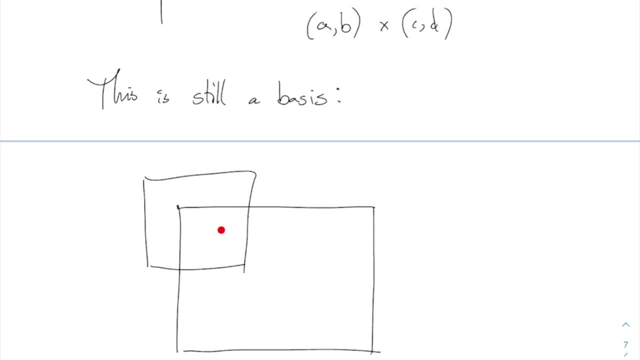 can you make a box inside the intersection? Yes, Yes, Yes, Yes, Yes, Yes than the picture for circles. so the intersections property also holds intersections, all right. so the boxes make a basis and so we can define a topology using the boxes. so there's like the standard topologies when you use circles for. 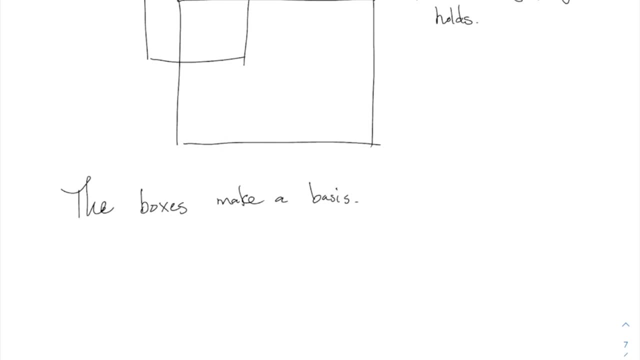 everything. what if, instead, I use little rectangles for everything instead of circles? it turns out these boxes also generate the standard topology, that is to say, if you think about sets being open in terms of rounded neighborhoods, those same sets are automatically open in terms of boxy neighborhoods. it 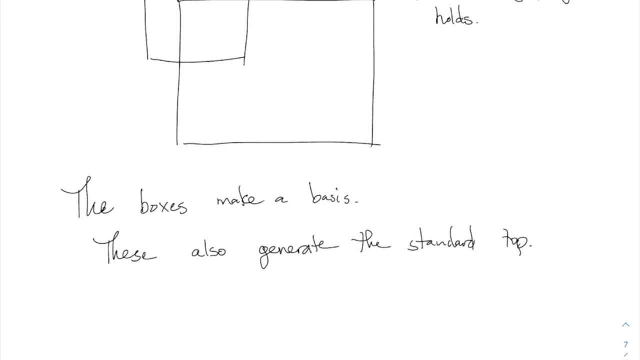 doesn't make a difference if you're using circular neighborhoods every time or rectangular neighborhoods every time, for example, all of those sets that I said that we looked at before. if you have this set here and I asked, is it an open set in terms of boxes? it means can you put a little box around that point. 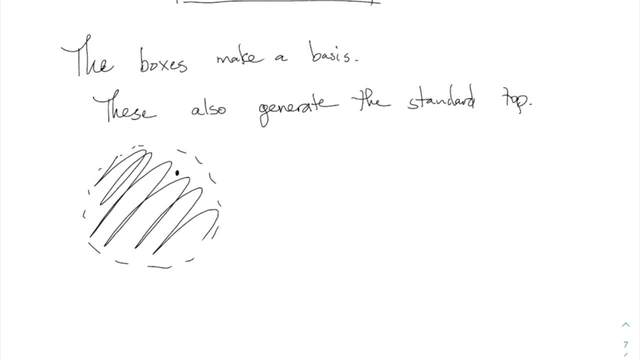 inside the set, but the answer is still yes. I mean, you can make a little circle around, but you could also, if you want, to make a little box around it. so this is, I would say, still open, even if you're using boxes right or something like this. the triangle was the second picture. I do again, this is still. 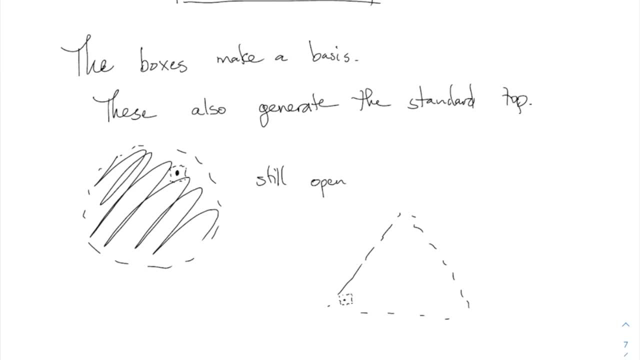 open. there is, every point has a little box around it. yeah, it's true, the center. yeah, these are boxes with sort of a side length of 2 epsilon or something like that. if you like, it's true, but it doesn't matter. yeah, all that matters really is like, can you put little boxes around any point? and the answer is like, really, if you? 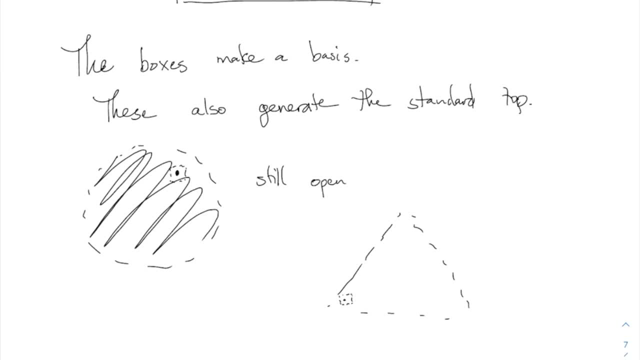 could put a little circle around it, then you could also put a little box around it. and if you could put a little box around, you could also put a little circle around it. so the distinction is irrelevant. so our book actually does. another example: we can generate the standard topology. 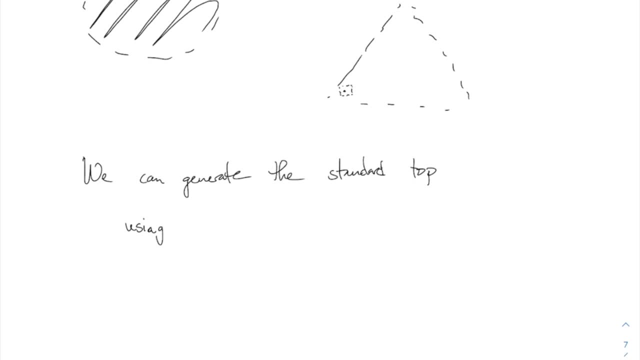 using any kind of- i don't know about any, but any kind of little shape that you like. so you can use little circles, if you want to, or you can use little boxes, if you want to. you can get the same topology when it comes to using these to define neighborhoods. it generates the same types of open 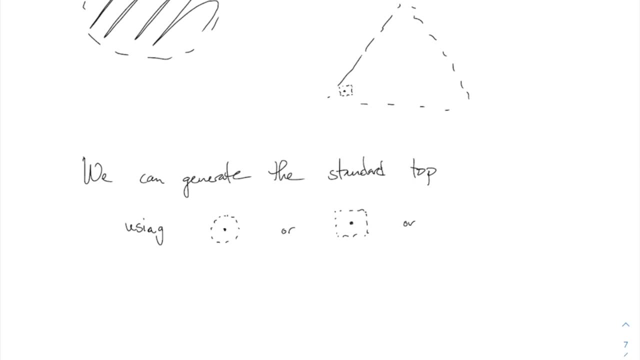 sets, or i thought this was cute. in our book he, they specifically say: you can use a little heart shape. why not? it doesn't matter really, whatever the shape looks like, as long as that shape is something that you could shrink down as far as you like. right, this is the circles or the boxes, or the 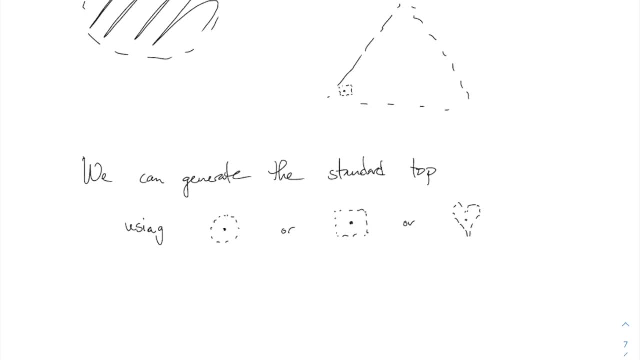 they all generate the same topology in the end, and so what that means is this is kind of good news. it means that we can use whichever one is the most convenient. so if you don't like using the euclidean distance formula- which i don't really because it has a square root in it- you